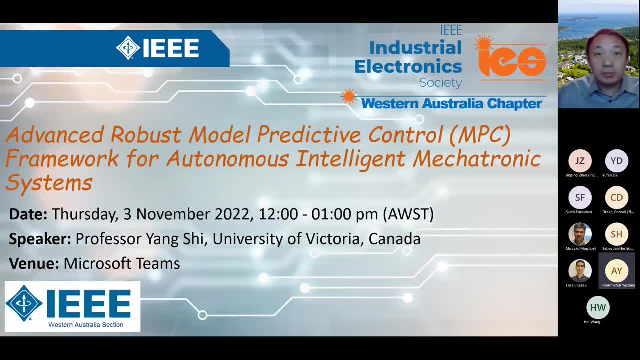 His current research. His current research interests include networked and distributed system model, predictive control, cyber physical system, robotics and mechatronics, navigation and control of autonomous systems and energy systems application. He is the vice president of the conference activity IEEE IES and the chair of the IEEE IES Technical Committee on Industrial Cyber Physical Systems. 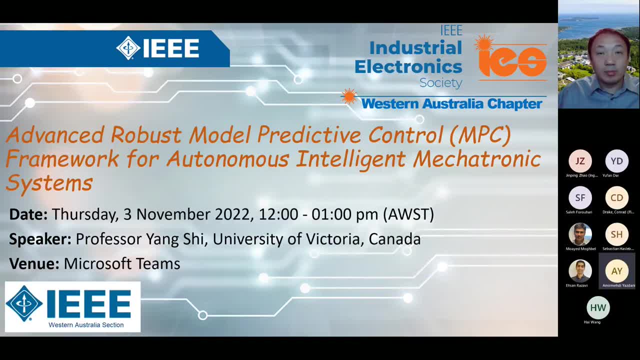 He is the vice president of the conference activity IEEE IES and the chair of the IEEE IES Technical Committee on Industrial Cyber Physical Systems. Currently, he is a co-editor in chief for IEEE transactions on industrial electronics. He also serves as the associate editor for Automatica, IEEE Transaction, Automatic Control and so on. 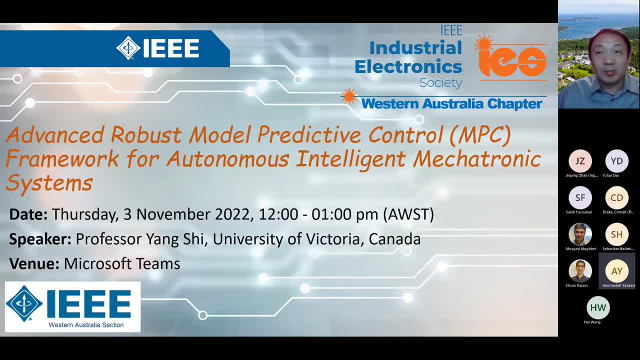 Okay, it's again our pleasure to have Professor Yang Shi. If you are ready, the floor is yours, Thank you. Thank you very much for the very nice introduction and thanks for the invitation. So, just in case of any network congestion problem this morning, I recorded my presentation. 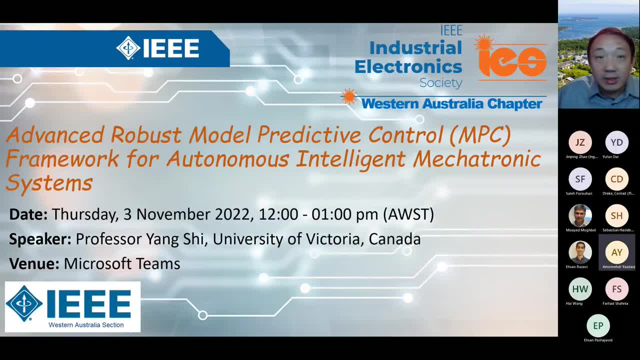 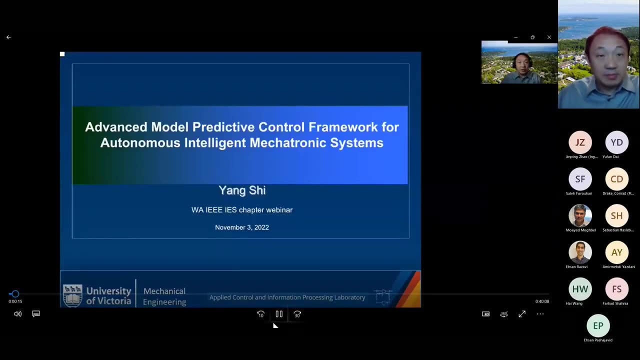 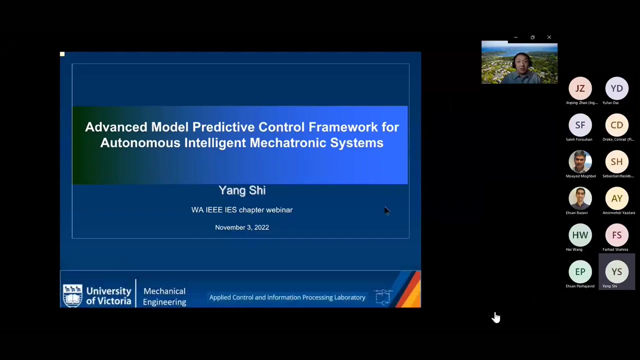 So I'd like to share my screen right now. Thank you very much. So give me just one second: This presentation online. So today. good afternoon everyone. Thank you very much for attending the webinar. It's my great honor to be invited by the Western Australian IIIES Chapter to give this presentation online. 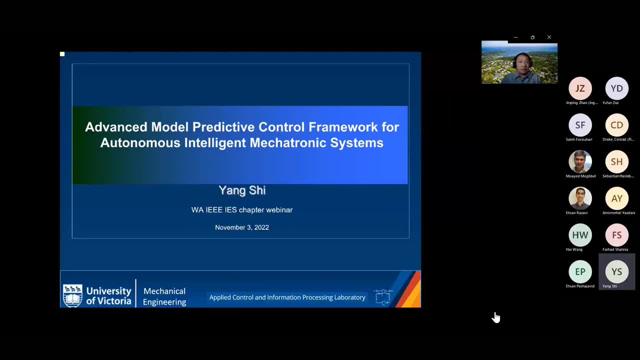 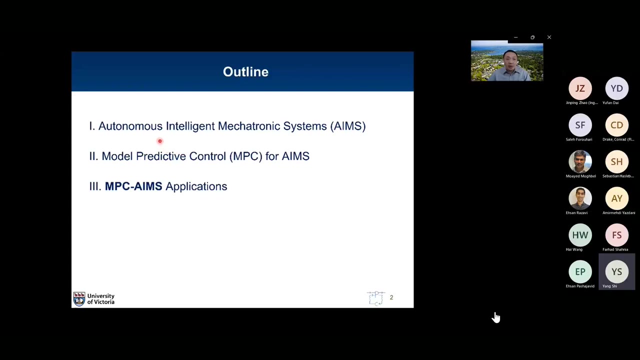 So today my talk is on Advanced Model Predictive Control Framework for autonomous intelligent mechtronic systems. So I will first briefly introduce the main design challenges about the AI-MS- autonomous intelligent mechatronic systems- in general and then point out and summarize some 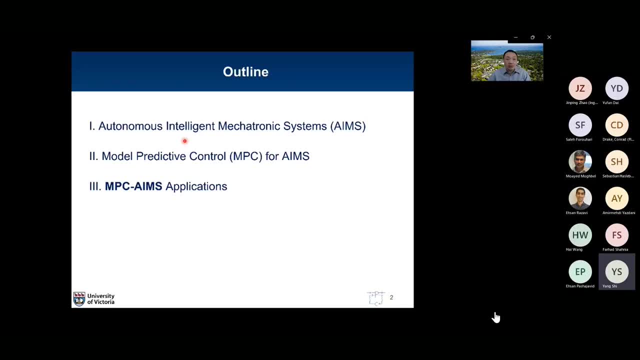 especially the challenges from the controls perspective. And then I'd like to propose to design the multiple data control for the applications of AI-MS. And in the last part I mainly introduce several of the recent applications of MPC to advanced autonomous intelligent mechatronic systems. 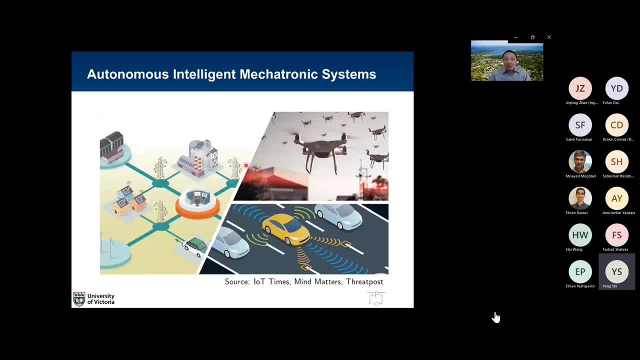 So we see that in many of the applications, including the Internet of Things or industrial cyber-physical systems, autonomous vehicles, autonomous vehicles and unmanned autonomous vehicles- or driving and smart grid. so large-scale smart grid or large-scale cyber-physical systems. 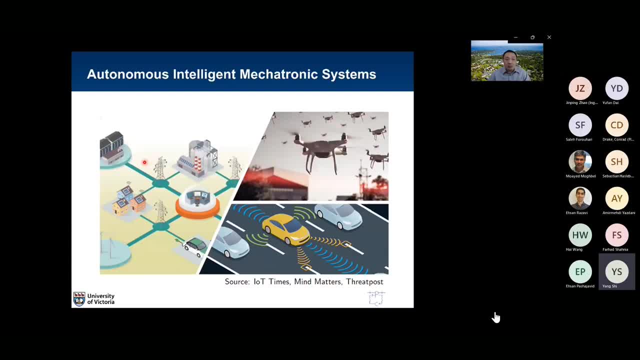 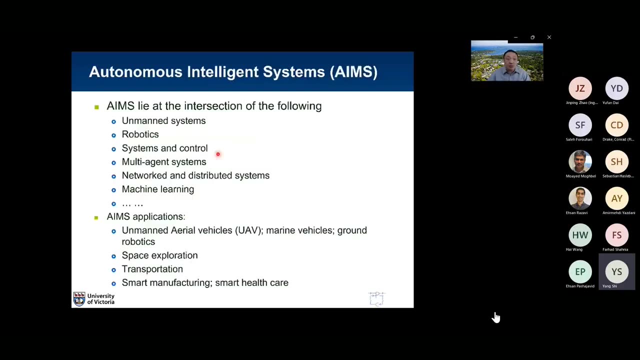 we can always find the specific applications of mechatronic systems. In other words, mechatronic systems are actually playing a fundamental role in building up a large-scale cyber-physical system. So specifically, AI-MS lies in the intersection of the following disciplines: 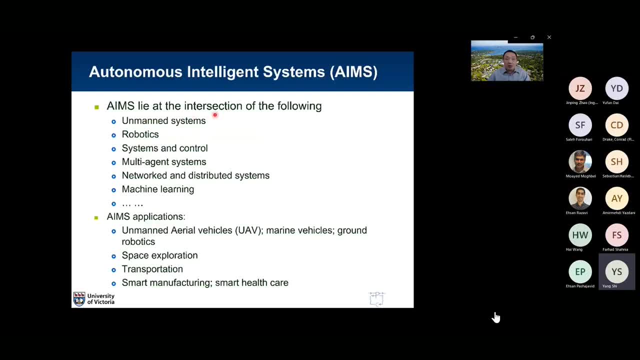 including the application requirements from unmanned systems, remote and autonomous. We can also find requirements from unmanned systems, robotics, and also from the theoretical study areas, including system and control, multi-agent cooperative control systems, network and distributed systems and machine learning, and so on and so forth. 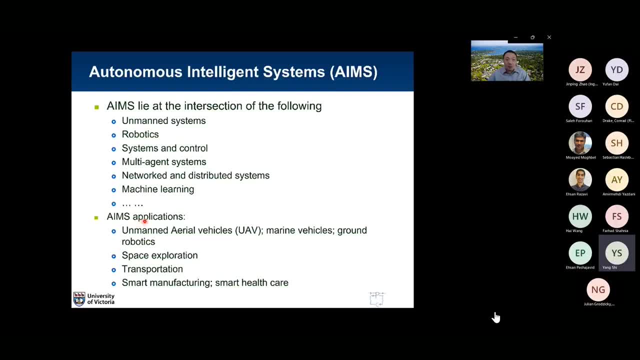 So mechatronic system can find broad applications in unmanned aerial vehicles, UAV, marine vehicles, ground robotics, space exploration, smart grid and so on. So mechatronic systems can find broad applications in unmanned aerial vehicles, UAV, marine vehicles, ground robotics, space exploration, smart grid and autonomous vehicles. 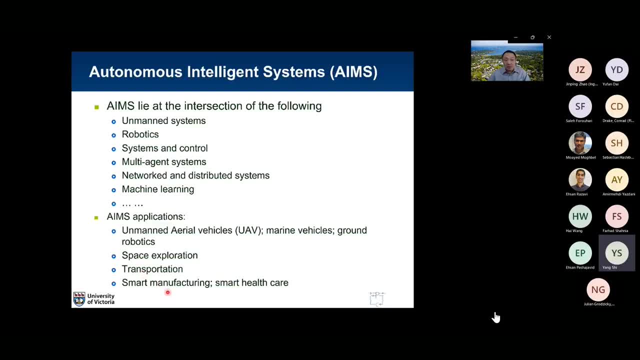 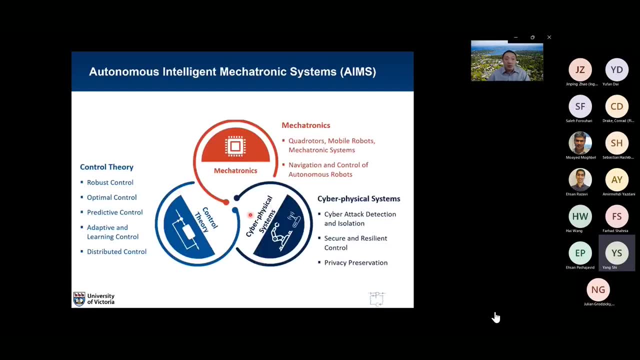 and smart grid, and also in unmanned aerial vehicles, the robust overall operating organization, smart transportation manufacturing, additive manufacturing, smart healthcare systems. So, in order to develop the autonomous intelligent mechatronic systems, we need to study not only the theoretical features. 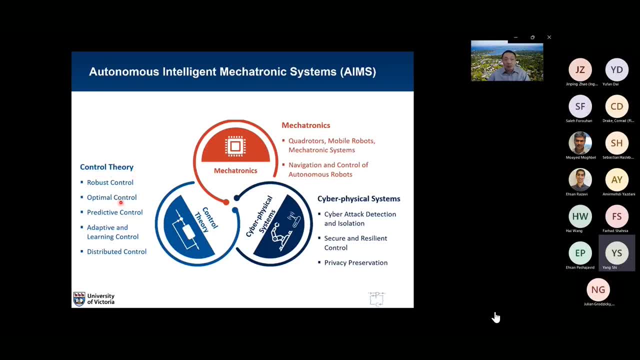 but also some application consideration. So, in terms of control theory, so many of the control strategies have been successfully applied. applications: In terms of the application, the mechatronics system has been applied to develop the quadrotors, mobile robots and some other type of autonomous vehicles, And we need to consider 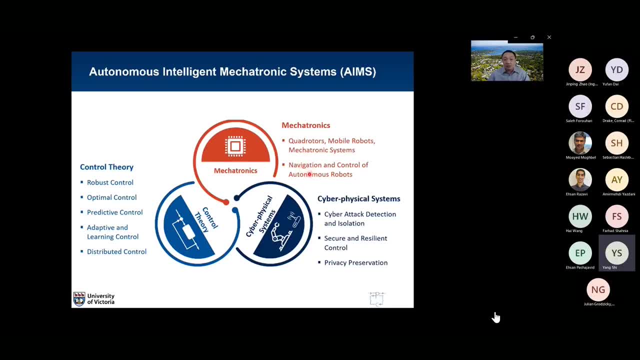 the design of the navigation and control of these systems And further many of the small-scale mechatronics systems being integrated together, they can build up the cyber-physical system called CPS. So within the CPS relative larger scale, we need to consider the cyber attack detection. 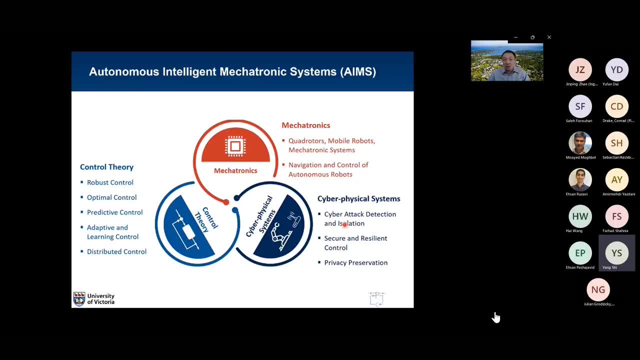 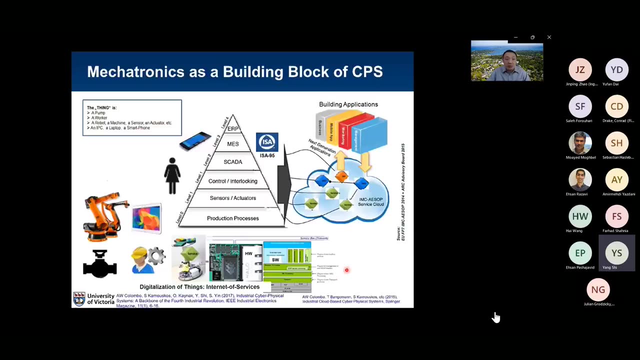 and isolation, leading to the fault-tolerant control, secure and resilient controller design and how to preserve the privacy. So this tends to be a very important consideration in the nowadays cyber-physical system development. So, looking into the ISP standard- ISA 95, so this gives us a big picture of a cyber-physical system. 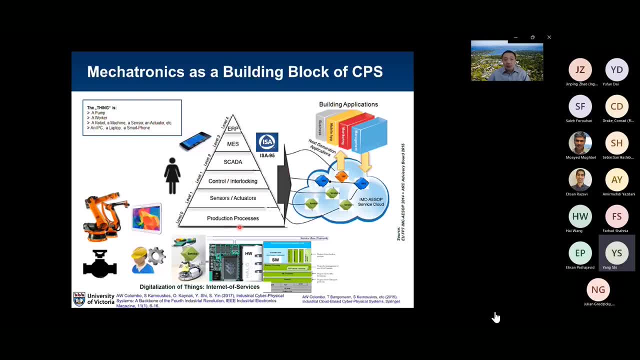 It consists of the lower level production processes and further sensors and activations, control system design and interlocking. And to the upper level we see the application of the SCADA systems or even the larger scale MES and ERP design. So again within this cyber-physical system development, 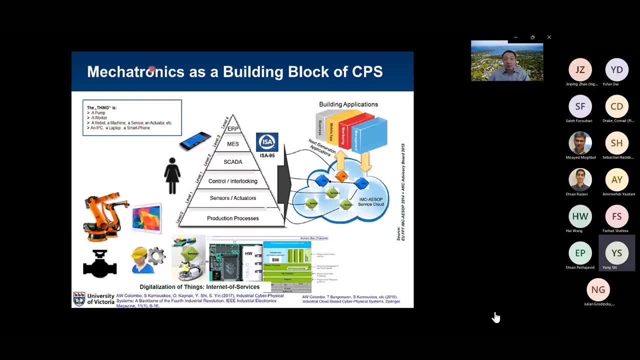 So everywhere we will see the application of the mechatronic systems. So mechatronic systems are playing a building blocker role in building up a large scale systems. So they are also referred to many of the possible things, including the closed loop system, small scale. 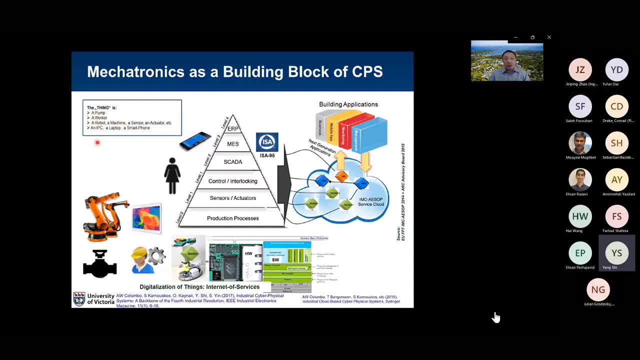 a pump, human worker, robot machine and laptop controller or microcontroller, or even the smartphone as a device. So if you are interested in more details of cyber-physical systems, you can refer to the research book published in 2015,. 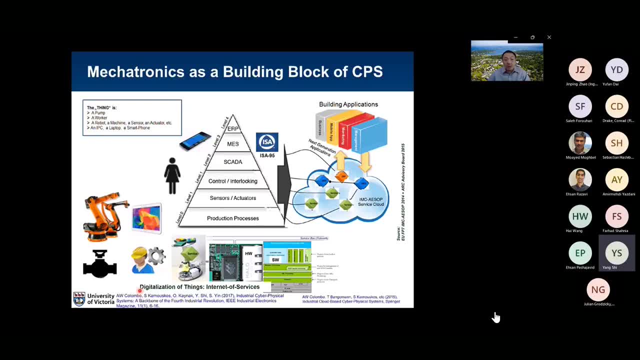 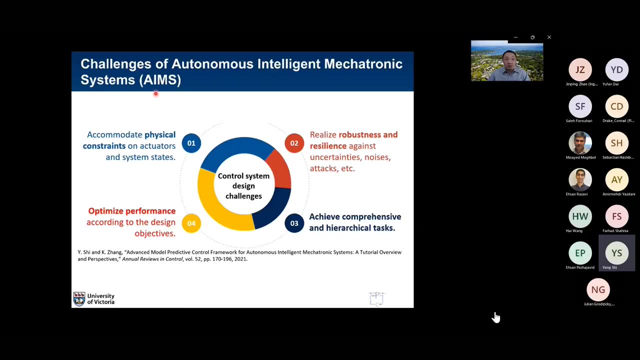 and a recent survey paper or prospective paper, published in 2017 together with my colleagues in HP Industrial Electronics Magazine. So, but today we're going to focus on how to consider the design challenges of AI-MS and then we can clarify, you know. 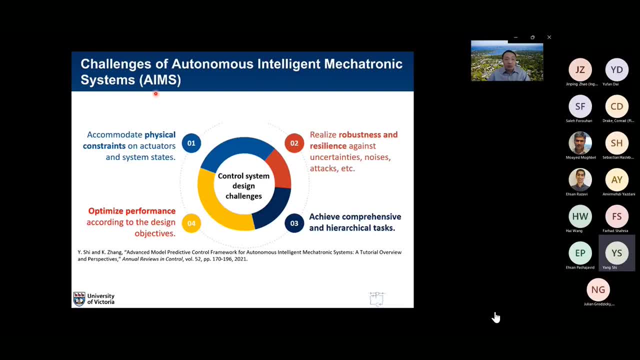 how to look for a most suitable control strategy to deal with the control system design for enabling the application of AI-MS, So number one in order to control a mechatronic system. so first of all, we need to consider accommodating physical constraints. 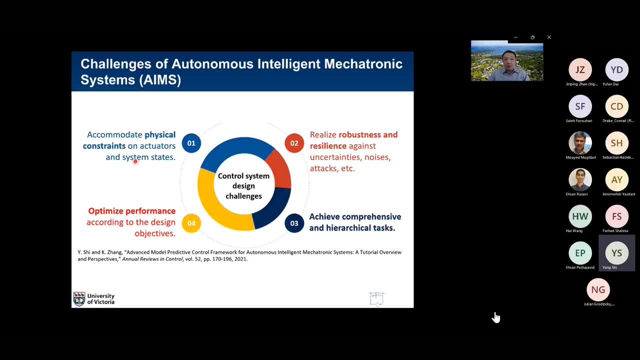 not only on the activity but also, you know, on the application of AI-MS, But also on the involved system states like the velocity, acceleration or even temperature of a dynamic system. Number two: we need to realize the robust control. 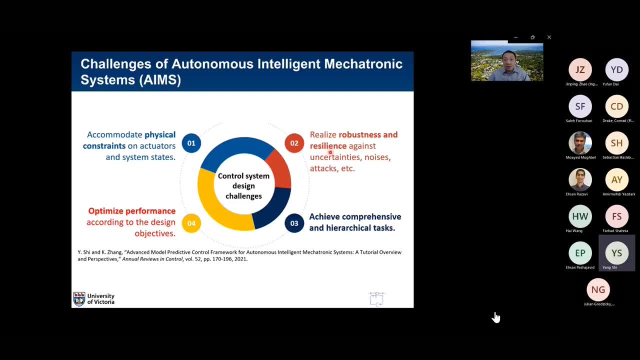 and also the controller should achieve certain level of resilience against unknown uncertainties, noises and even cyberattacks. Number three: we need to design our controller for the mechatronic rate electronic system in order to achieve comprehensive and hierarchical tasks because, in order to operate, 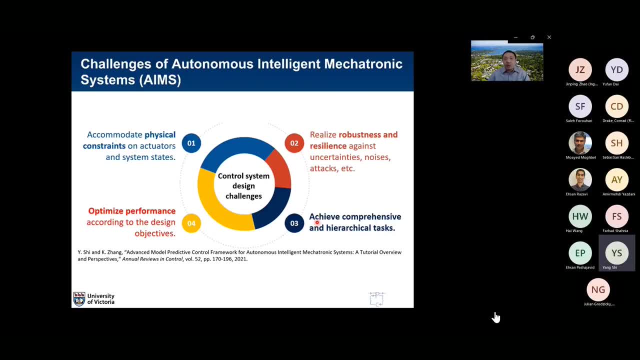 and run any type of autonomous vehicle. so the mission and the tasks will be of the comprehensive and hierarchical feature, including the high level cost planning and obstacle avoidance and further the tracking or pass following or dynamic positioning. so we actually need to consider how to realize this. comprehensive tasks. and number four, finally, we aim to achieve certain 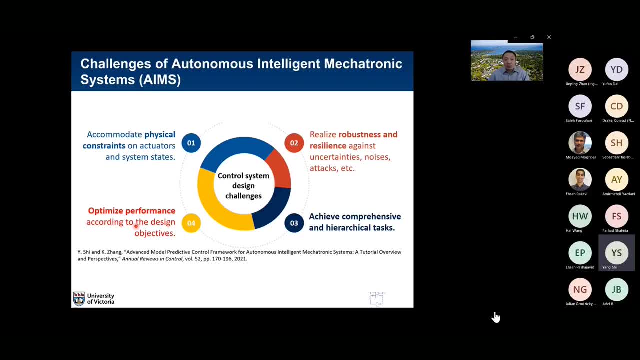 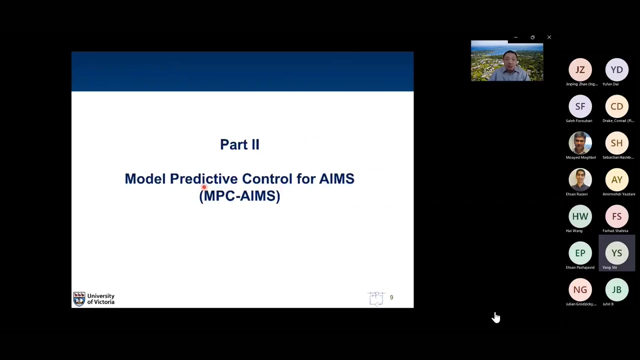 level, optimal performance according to our proposed design objectives and the tasks, so summarizing all the expected outcomes or or features of the controller design for electronic systems. we need to proactively look for a appropriate control strategy to design the controller. so in here our objective is to develop a very unified control framework for dealing with the 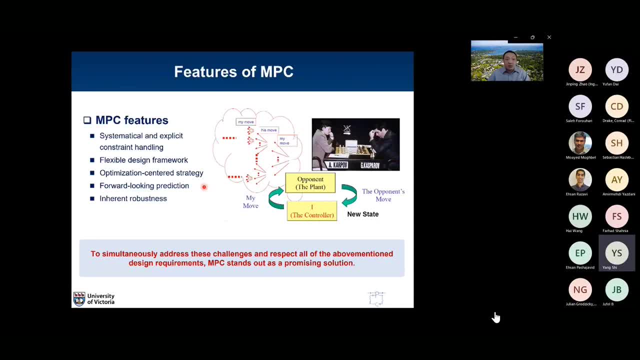 control system analysis and the synthesis of its controller system design. so in this case, considering the expected features that the controller for electronic system should have, model predictive control stands out as a quite promising solution. so this is mainly due to npc's very attractive features. so first of all, it can very systematically and explicitly handle all the 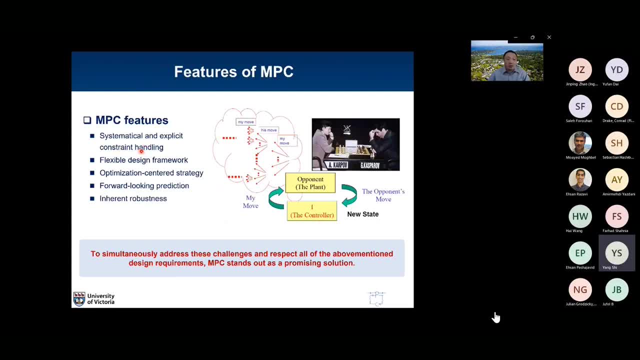 physical constraints. that's exactly corresponding to the first requirement of electronic system control, considering the control input saturation, considering the state constraints in real time. and secondly, npc provides a very flexible design framework, which will be discussed very soon, in a few seconds, and npc is actually optimization center strategy and therefore it naturally provides 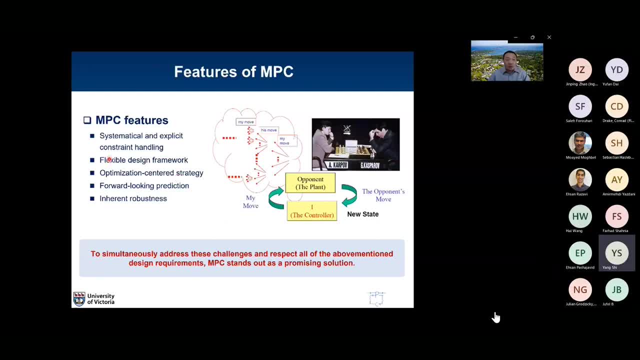 the suboptimal or optimal performance, and npc provides forward-looking prediction. so this feature can enable us to tackle many of the design challenges that will be encountered in electronics or motion control system design, and also npc does provide the inherent robustness and let her know we 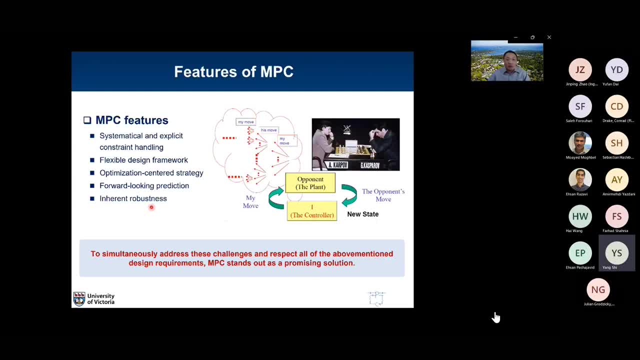 need to proactively design the robust control for enhanced robustness, but naturally npc itself already has certain level of inherent robustness. this is exactly what we want in designing any type of electronics control systems. so there is a very natural analogy between the chess play and the 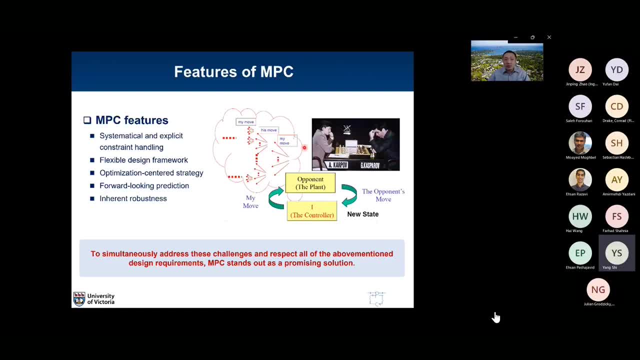 npc strategy. so just a few words on the chess play. any player will do the prediction in their minds, not only producing the current strategy to move the uh to move, to make the current move, but also they'll make some future predictions and then, at the current time, the player will just 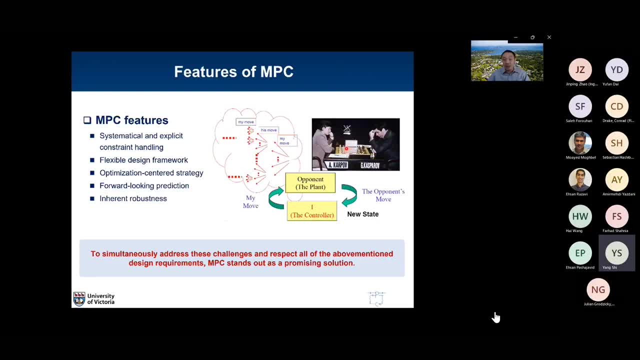 make one move in this uh, in this, in his turn, and then further it will turn to the opponent's uh decision and then this opponent chess player will be very fastly running in his mind certain type of opposition based on the observed, the current situation scenario, and then making a decision. 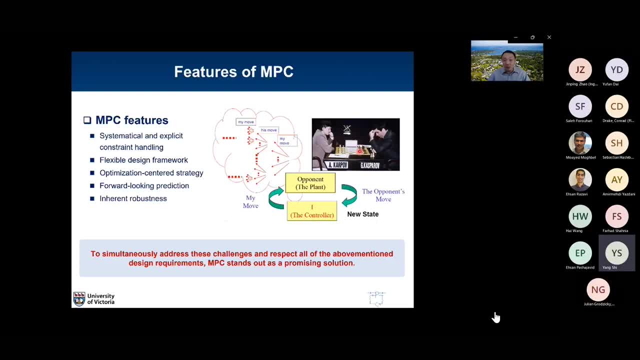 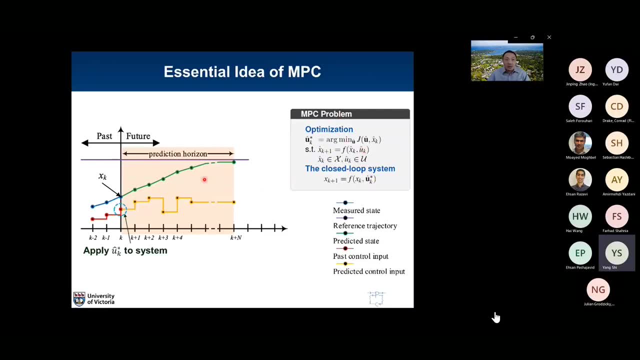 including the current move and also some predicted moves. so this is exactly what model predictive control will be doing. so let's take a look at this dial one. at current time, instant k. so npc controller will run the optimization problem, generating a sequence of a control impulse. so 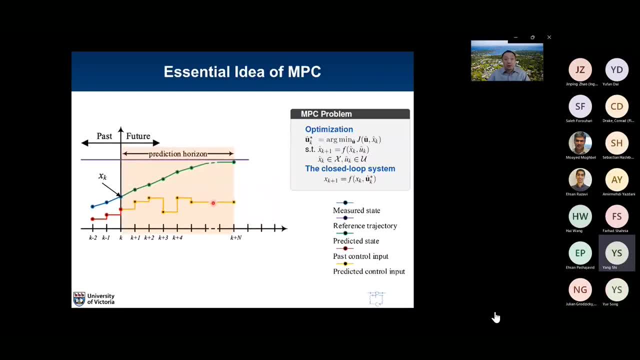 here, if we talk about the single input, single output, control, uh system, and then classical control strategies will just implement or and generate a current control input signal, which is a scalar signal, but npc, different from traditional strategies will be- will be generating a sequence of the control profile, which is a vector in this case, and then the signal to be sent to the activator. 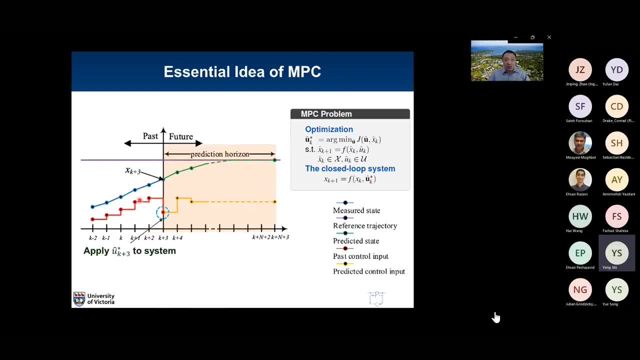 to implement the control input will be a scalar. that's the first element of this vector. so therefore, you see, at time instant k, a sequence of the control input profiles have been generated, but only the first time means that the intervals control input will be sent to drive the actuator. 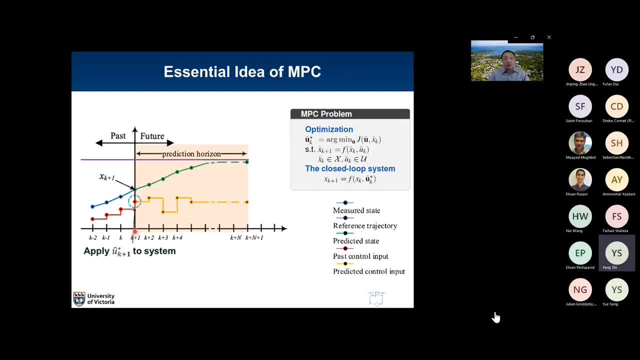 and then, moving to the second time, instant k plus one, the similar procedure of the of solving the optimization problem will be repeated. so the first segment, segment of the vector, will be sent and to the actuator and implemented. so therefore, model predict control is also called a receding horizon control strategy. so how to generate a control input of predictions? 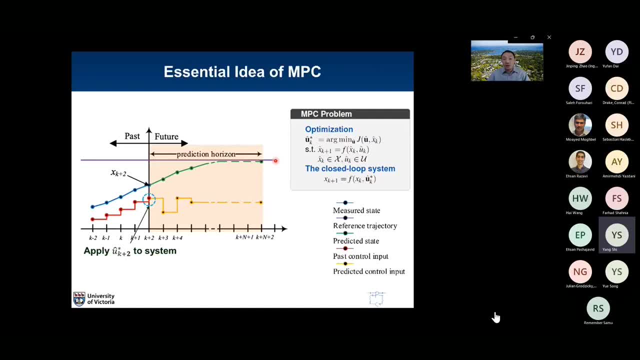 the, the vector or the profile. so this is generated by solving the formulated constant optimization problem. so you can see here: so state constant and control input constant can be very systematic and conveniently incorporated into the constant opposition problem, if the this constant opposition problem will be giving us a feasible solution. and then they generated the first element. 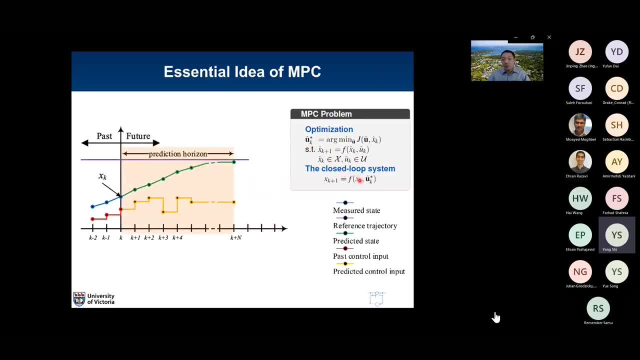 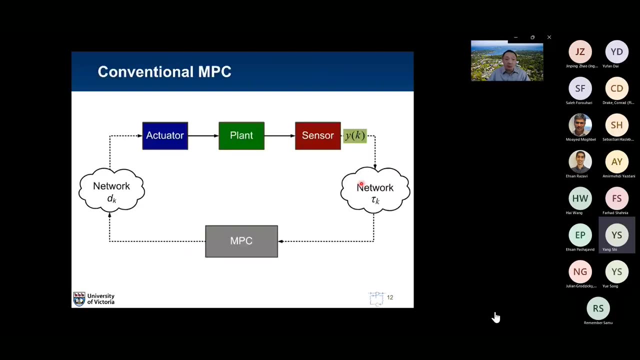 within this uk star will be sent to control the system leading to the closed-loop system and then all we need to analyze is to figure out under what conditions the closed-loop system will be stable and to certify some other required features and characteristics. so you can take a look at this very classical control system background the sensor will be. 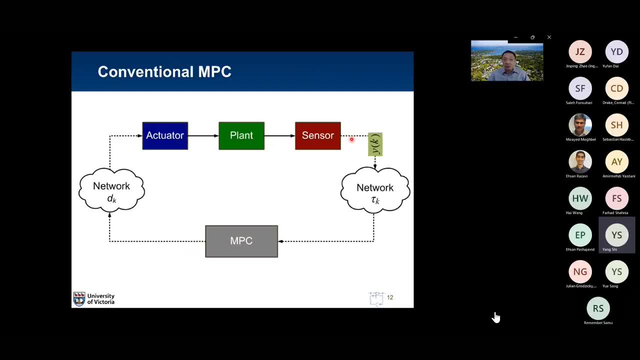 measuring some states of the dynamic system, transmitting the signal over the internet to a controller. so this controller will be solving the formulated optimization problem, generating a sequence of control input profile not only for the current time- instant, but also making a prediction for for next time you stand for next, next time instant, and so on so forth, depending on 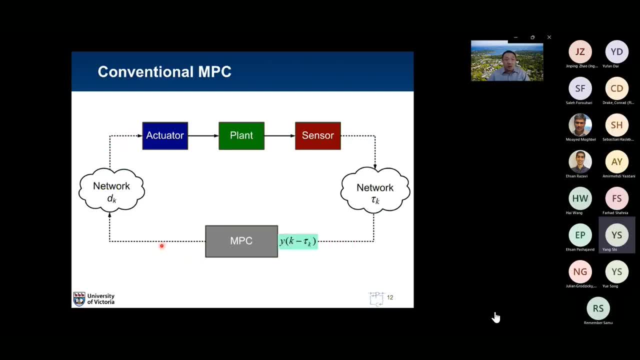 the prediction horizon we specify in advance. however, even though this multiple controller generates a control profile which is a vector for this single input, single output scenario, but only the first element will be sent over the internet to the actuator to drive the to drive the system. so this animation diagram clearly shows how conventional, classical, multiple control actually 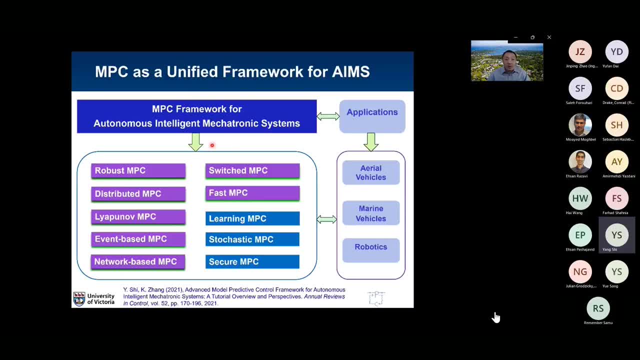 works. so we've been in the field with the virtual reality and the biomechanical technology for many years. we have been striving to producing and, you know, conducting research on proposing an npc framework for autonomous intelligent electronic systems. in order to achieve this on the theoretical side, we need to solve many related theory problems issues. for example, we need 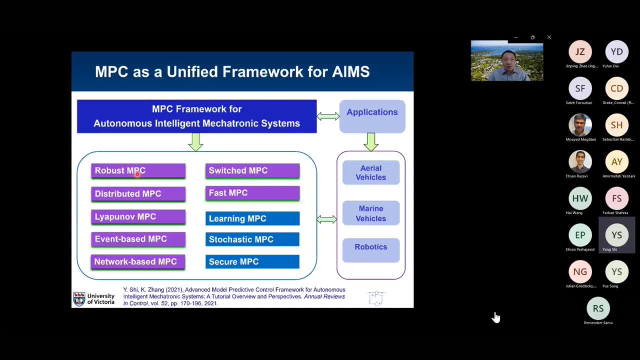 to design robust npc to proactively consider the avoidable uncertainties, noises, And we need to design the distributed MPC for a large-scale interconnected dynamics or the multi-agent system, For example, if we have a group of drones working together, cooperatively flying. so how to design the distributed strategy in terms of 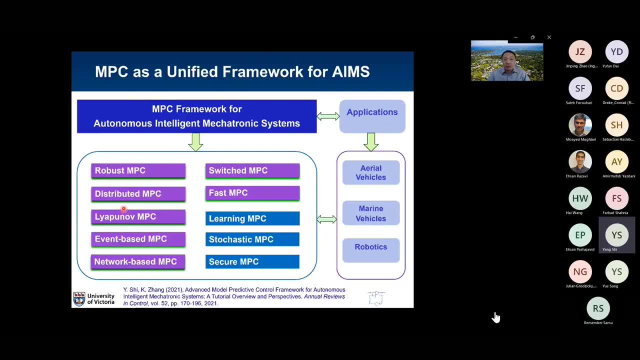 mobility control And we also studied the theoretical as Neapolitan MPC, primarily aiming to ensuring the stability of the closed-loop system And further, in order to reduce the computational complexity and also the communication load, we studied the event-based MPC, meaning that 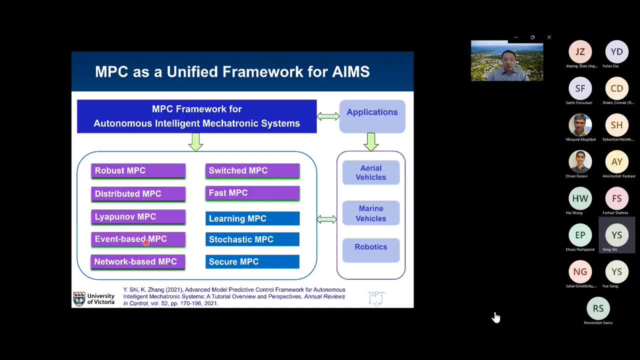 instead of periodically conducting the optimization solving the model productivity control, optimal problem, optimal control problem- we can actually run and trigger the solver to to tackle the optimal control problem a priori, Depending on the needs. we never need it, we just trigger the controller And then, if we not need it, we can let the controller to have a rest. 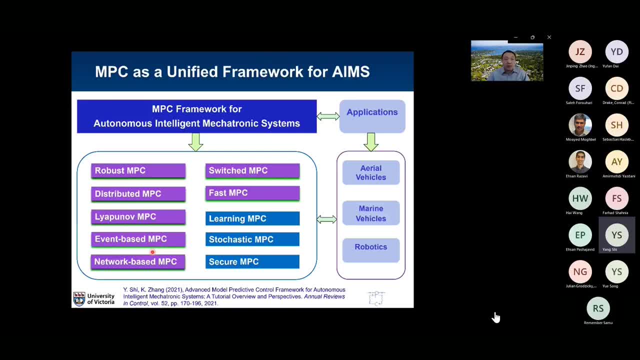 So this can greatly reduce the computational complexity and also save the limited bandwidth for not transmitting information periodically. So this is called event trigger control and the control of the MPC. the end user-dominated MPC is a type of MPC that can be used to trigger the control of the MPC or the self-trigger control. So also we have developed a theory on 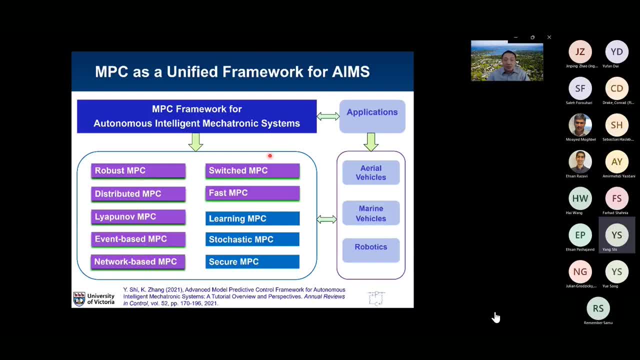 network-based MPC considering how to tackle the network-induced constraints like time delays, packet dropouts and so on, And switch the MPC because many practical systems are actually operated in terms among several different modes or different mac model of using. switch the dynamics to characterize your practical system and the 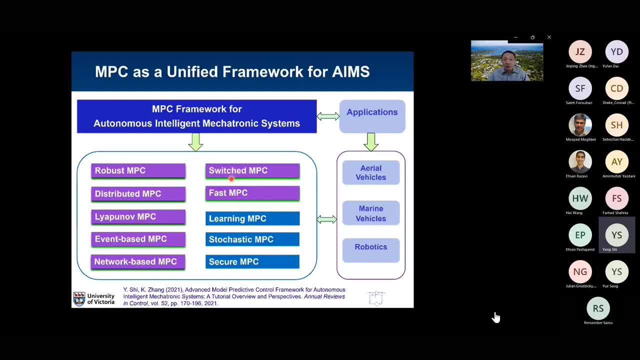 overall mission completion. so therefore, we need to design the theoretical switched npc strategy for such a type of a system and, more importantly, we need to consider the design of the fast algorithms to achieve the real-time implementation. so just just imagine if you're going to implement the model productivity control to the motion control of a robot and then the sampling period. 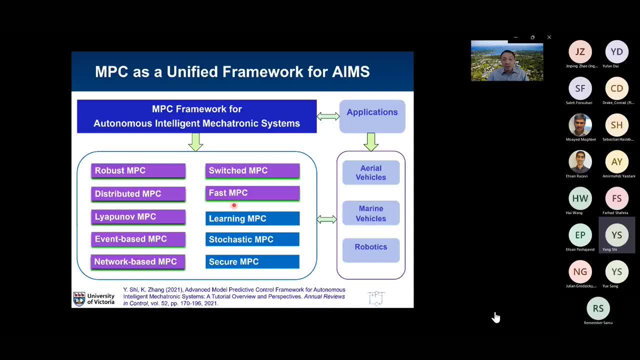 can be as small as a 0.1 second or 0.01 seconds, so therefore it does require the optimal control problem to be solved within such a short period of time. otherwise a real-time implementation cannot be successful. and if we consider the new application, 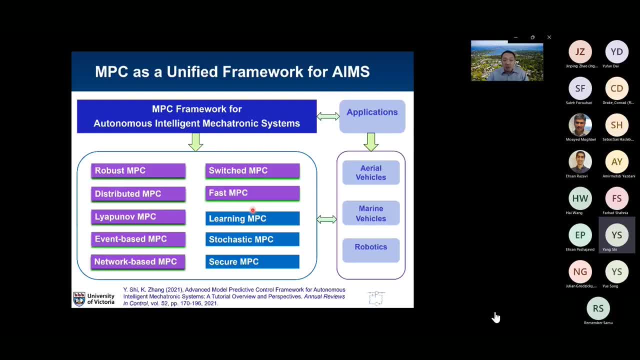 in which case the mathematical model is not always available or the mathematical model will be subject to some uncertainties or parametric uncertainties or unknown parameters. so in this case we need to develop the adaptive and learning npc and further, if we consider some stochastic environment, like you know, the constraints will not be, or with the hard constraints, 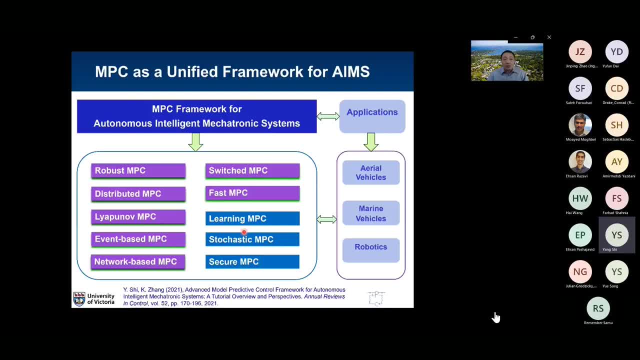 so sometimes the the constant can be characterized by probabilistic sense, so in in worse. so, if the constant can be satisfied with, you know, 95 percent- and then this naturally needs to a setup called stochastic npc scheme and secure npc. uh is very important for applying npc to large scale systems. uh in this type of physical system setup because cyber. 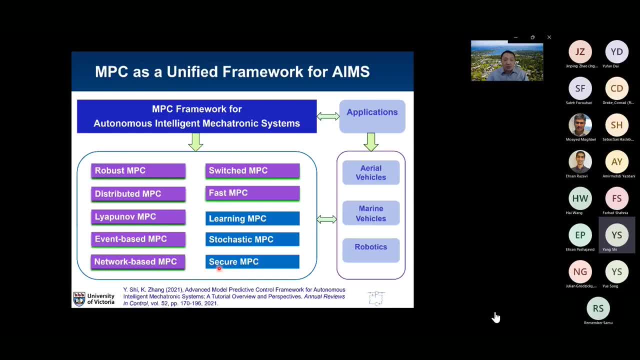 attacks will be a very important issue we have to consider. so putting this all together, so by solving this theoretical issues, we can possibly apply the appropriate the npc schemes or strategies algorithms into a specific application, including aerial vehicles or drones or a group of drones for multiple, multiple agent systems and marine vehicles or autonomous surface vehicles. ground: 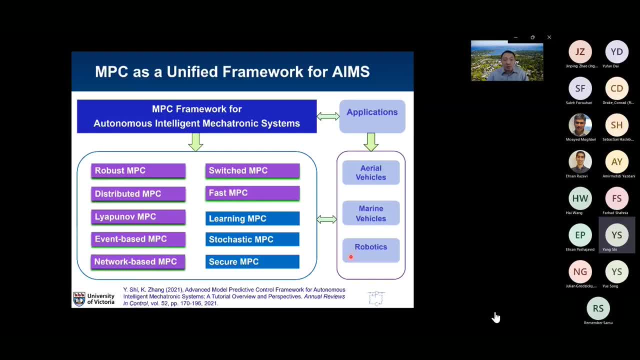 robotics and some other type of robotics applications. so, in order to apply npc to the aims system, we need to have a strong support from the theoretical research and, specifically, in order to apply the algorithm to control a real-time system, we need to make a very good combination of several of these strategies together to achieve our objective. so let's. 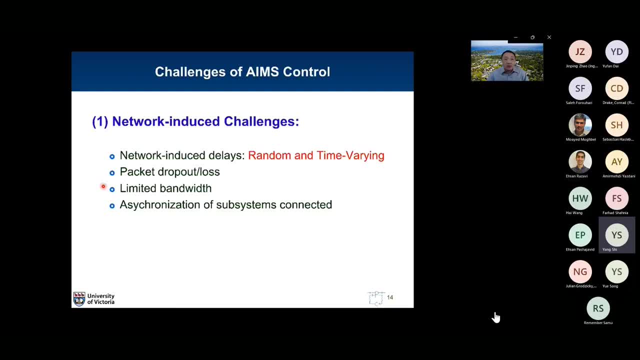 take a look at some of the challenges we have to consider when designing the npc for electronic systems applications. so number one: many of the mechatronics applications nowadays are actually placed and operated in a network environment, so therefore the network induced constants must be considered and compensated first. it comes from the random time delays. it's time varying. it's random. 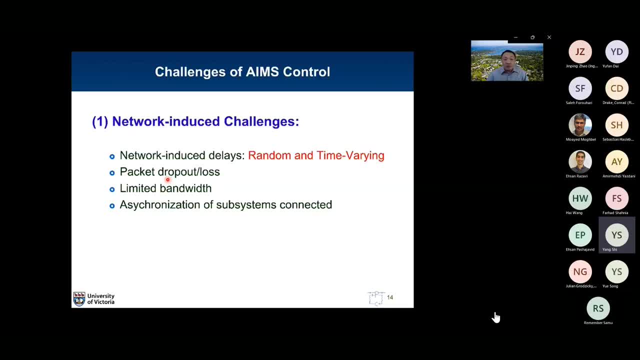 and we may also suffer from the packet dropouts, and this will be occurring in a random style. be careful also when making a fix or some kind of하는데 to bending the platform, as the stress at the distance it can also be a common problem. so the information may be transmitted and may not be transmitted to the controller of the. 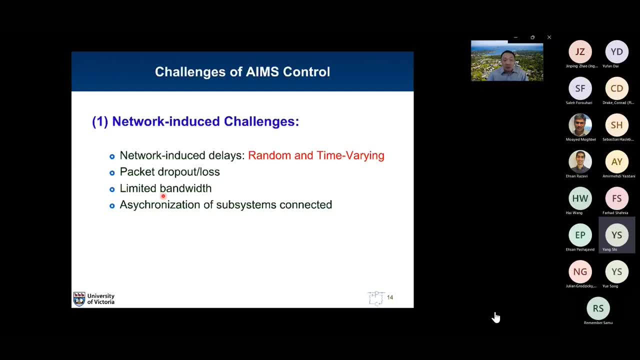 actuator in time and limited bandwidth because many of the information will be transmitted over the limited network. so, therefore, how to make full use of the very limited bandwidth to reduce? activators and microcontrollers are interconnected over the internet or the network, so the synchronization issue will be considered, because not all of 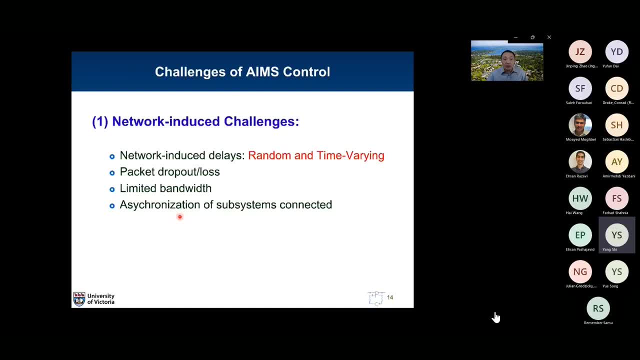 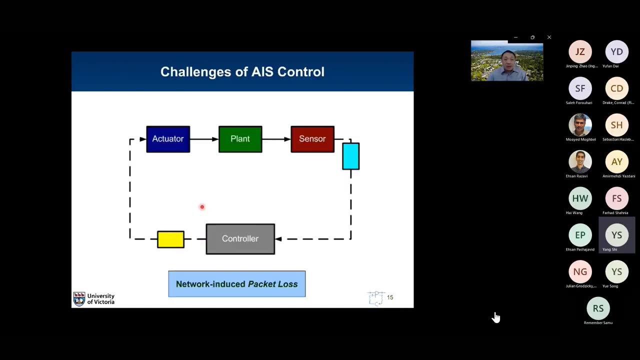 them are always a synchronized in terms of the unified clock. so in this case, if a synchronization would be the case, we need to consider the controller design to accommodate this possible a synchronization- and this shows the packet propose. so information may not be successfully delivered. so in this case, 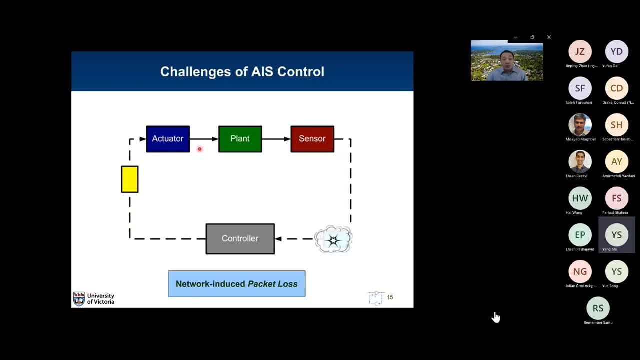 if the actuator does not receive the control signal, input or command in real time, and then the closed-loop system does not know how to work right. so we need to provide a very elaborated or dedicated a control system design for such application and, if the information can be delivered successfully, so it may. 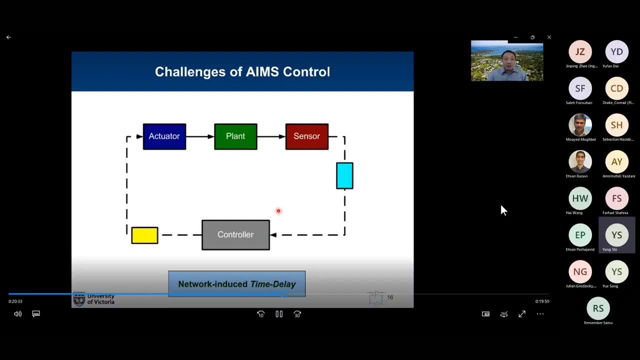 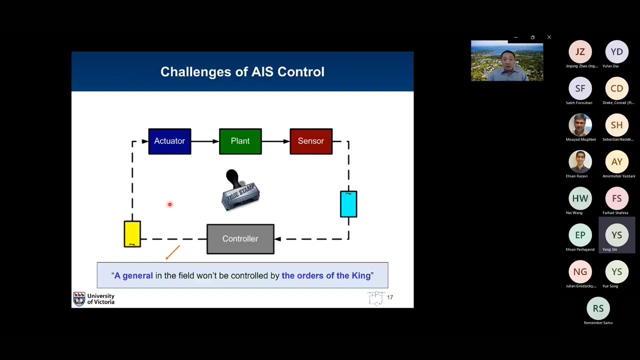 be subject to some time delay. we know that in control system. so even though the time delay might be minor or tiny, it still can degrade the control system performance or even make the system unstable. and we also comment that for dealing with the time delay or package dropouts from the sensor to the controller versus 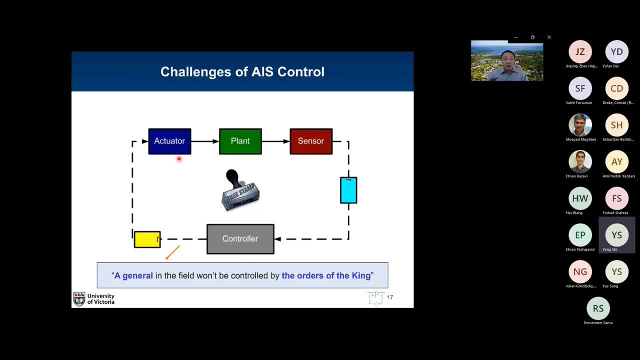 the time delay from the controller to the actuator, so they are different. so in order to compensate for both channel time delays, we need to apply different strategies. we need to develop a new type of methods to deal with the to deal with this as time delays in both channels simultaneously. 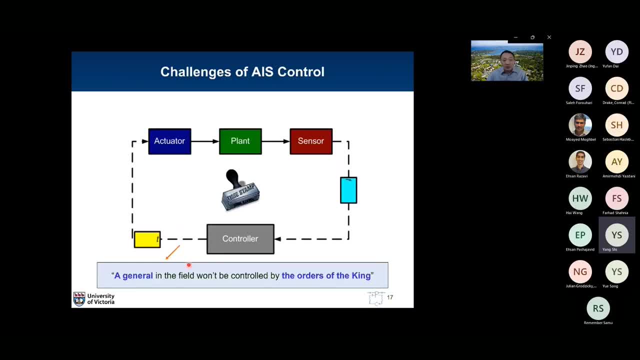 so here we quote a famous thing in China to describe why this left-hand side time delay from the controller to actuator will be so hard. or it will be even harder to be compensated because this time delay on this yellow block will be occurring after control system generated the signal. so in words, after the controller generates a control command. 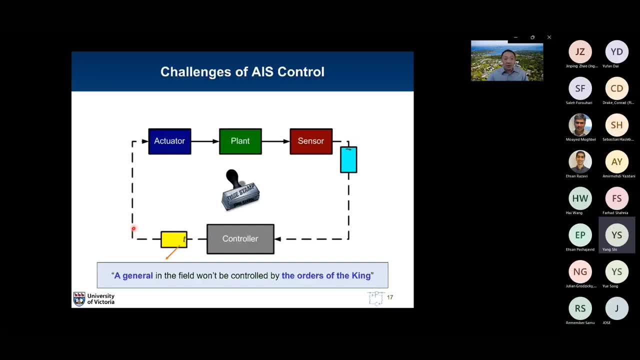 being sent out, the time delay will be occurring and observe afterwards. so therefore it's a it's not very easy to compensate this uh time delay that will be future generated. so same size. a general in the field won't be controlled by the order of their King, so in this case, so we need to. so in this case. so we need to do something that can do something that's similar. so some ways that a Då and the answer is one. I am so Again: yeah, and then at the next stage, trial will be somewhat paar degrees going on after this immediately, but we couldn't at least hot bleed them themselves. so in this, 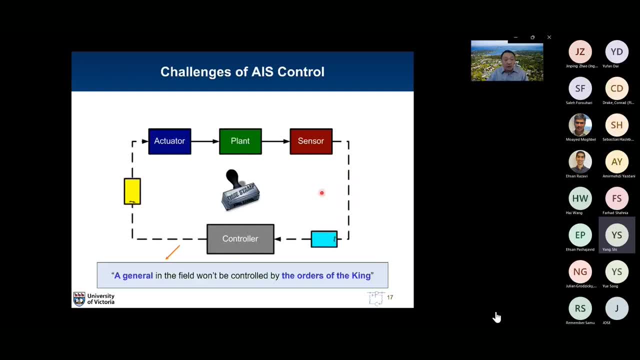 a The other data from last introduction, hogy at the first stage trial i have a fails Statement at, But i don't hope furtherƋthat it has been a problem 2016.. Men, you did 제가吧. that one was from the develop new methods to implement a very efficient compensation for time delay. number two: robustness. 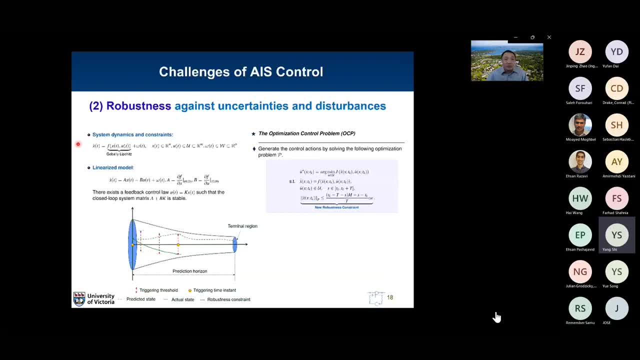 in any type of a control, no matter what kind of a control strategy we are going to apply for our applications in instrumentation, in control system, robotics and so on so forth, we always need to consider the robustness guarantee. so, generally speaking, robust control will consider under the 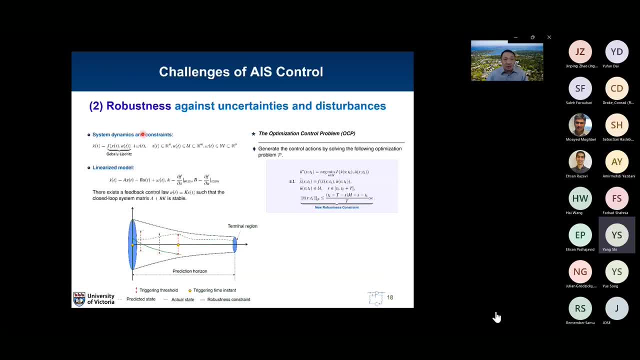 worst case of estimated uncertainties or disturbances, we still need to guarantee the performance of the design control system. so in npc application to the mectronic system we also need to proactively consider efficient, robust control, robust mobility, predictive control to guarantee the efficient robustness. so this is a one of the robust constraints. 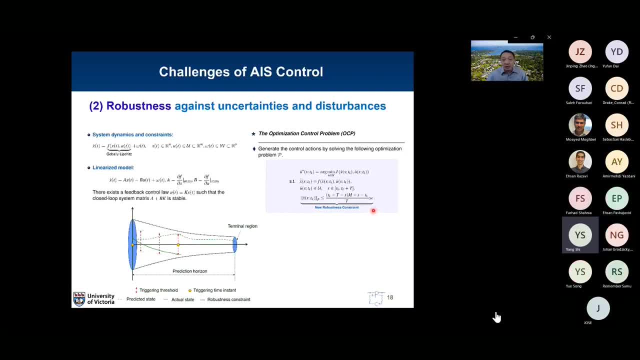 methodology we proposed several years ago and it's now becoming one of the important methods in designing robust npc. so it does have some certain conservative list, but it's quite easy to follow and it's easy to implement. it does not increase the computational efficiency and also it provides 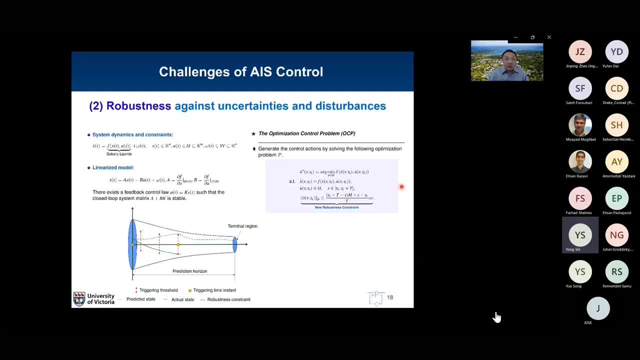 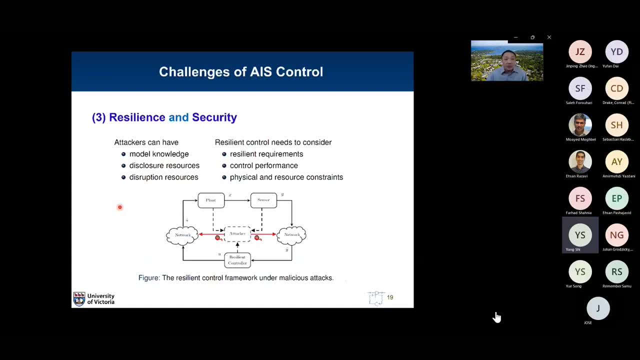 certain level of robustness to the design controller. and number three, in the cps applications- cyber physical system. so in the cps applications, resilience and security will be quite important because in any closed-loop system when we have the integration of the of the physical layer and their cyber domain, 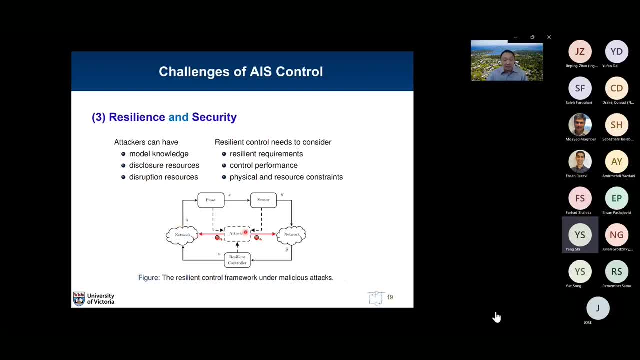 and then the information transmission might be subject to some cyber attacks, including dos, including the deception attacks or some other type of cyber attacks. so in this case we need to design the controller to achieve resilience and the security. so this is quite important for the current applications of a. 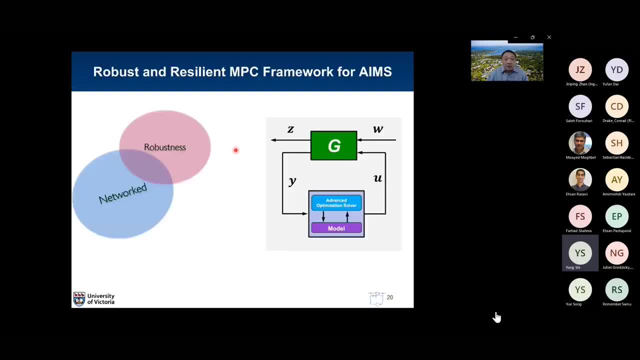 mectronic system. so, considering all the analysis. so our objective here is to design the robust and the resilient npc framework for autonomous intelligent mectronic system. so, keeping all the three key requirements in mind, we need to deal with this generalized uh system diagram by identifying the model as close as possible, as accurate as possible and 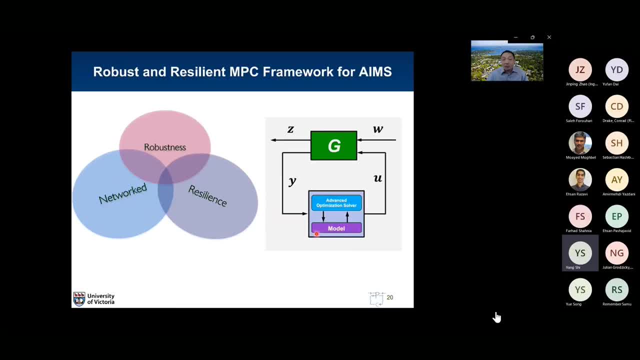 then, based on the mathematical model, we can develop the model predicted control as a unified strategy and framework and then introducing some advanced optimization solver to solve the formulated constant optimization problem, generating the control commands to stabilize or achieve the tracking control objective for mectronic systems. so within this generalized diagram, we have a lot of things to do. we need to. 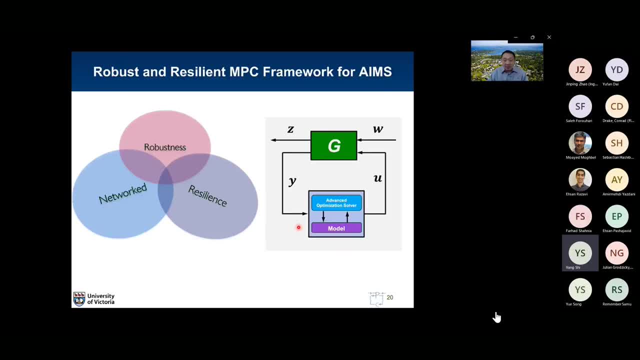 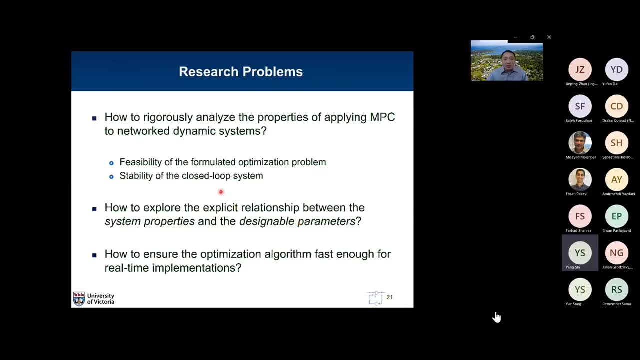 develop many algorithms to achieve our task. so, in general, we need to answer the following theoretical questions: so how to rigorously analyze the important properties after applying npc to the network, the dynamic mectronic systems, specifically including feasibility of the formulated optimization problem. so every time, instant, we're going to solve the optimization problem, constant optimization problem. 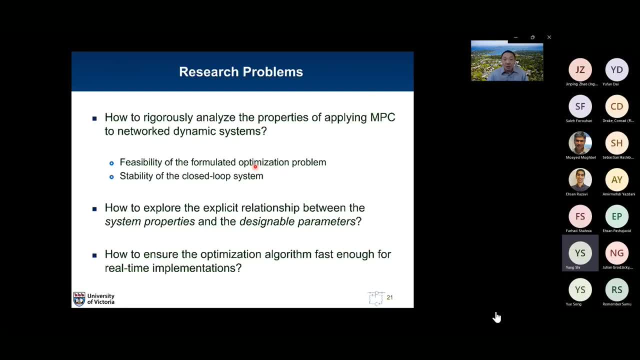 so how can we always guarantee this? uh, this optimization problem will give us a feasible solution. so this is the first question we have to answer and we have to guarantee uh, under certain derived conditions and if this problem can be answered. and then, second question, we need to. 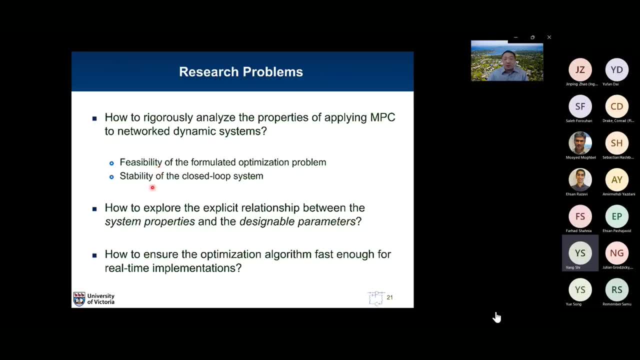 answer and address is how can we guarantee the stability of the resulting closed-loop system? and by this analysis we aim to develop the very explicit relationship between the system properties, as expected, with the designable control parameters. this will give us a guideline to choose appropriate parameter for real-time implementation. 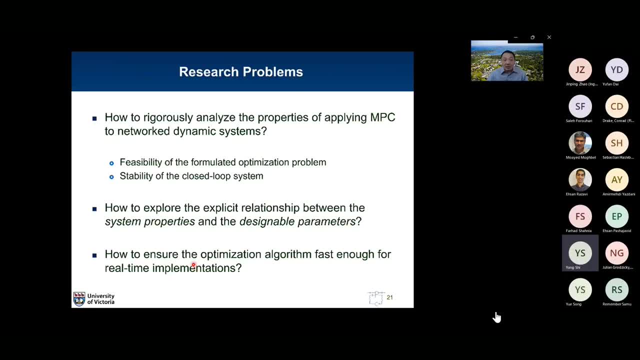 and last study. one very practical question we need to address is so: how can we assure the optimization algorithm firstly enough for real-time implementation in mectronics, because the in electronics, motion control requires the sampling period to be very small. so, simply speaking, we need to solve this optimization problem within the given short time period. 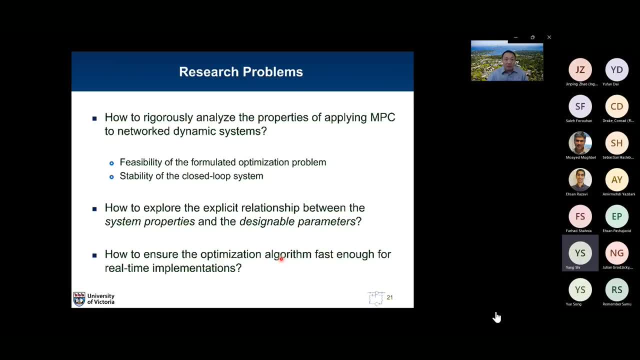 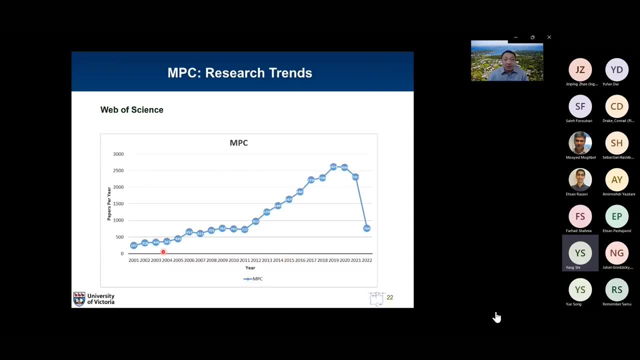 0.1 seconds or 0.01 second. so this is about the fussiness of the proposed algorithm. so in the past 20 years, if we make a summary of the publishing literature on multiple data control, so probably i missed some other literature because i only used the keyword npc to to do the search. 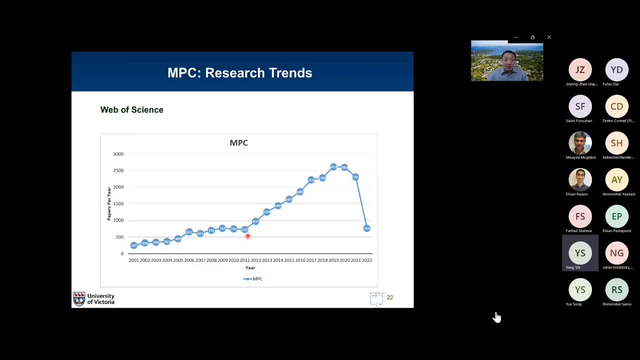 you can see very clearly, in the past 10 years there there was a sharp increase in the research trend of studying and investigating multiple data control and its corresponding applications. so let me report some of the representative applications of applying npc to mectronic system applications in my lab. so in 2017 we published two research books on: 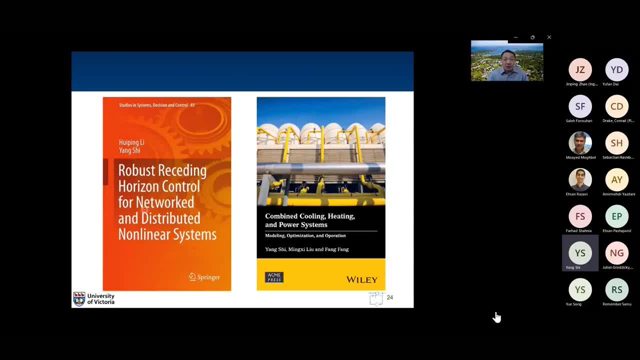 npc on the left hand side, robustly receiving or as a control for network and distributed nonlinear systems. so this is the first book on npc, for specifically network and distributed dynamic systems, and the second one it's on the application of advanced control and operate optimal operation for combined 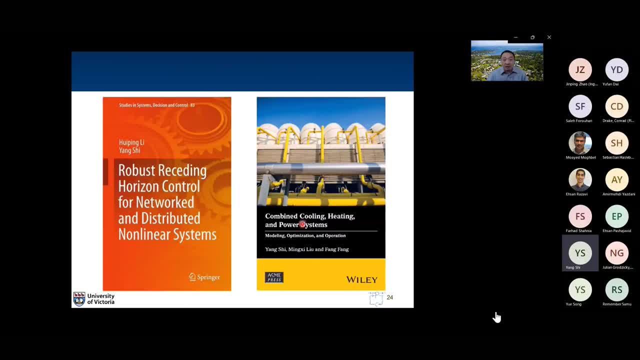 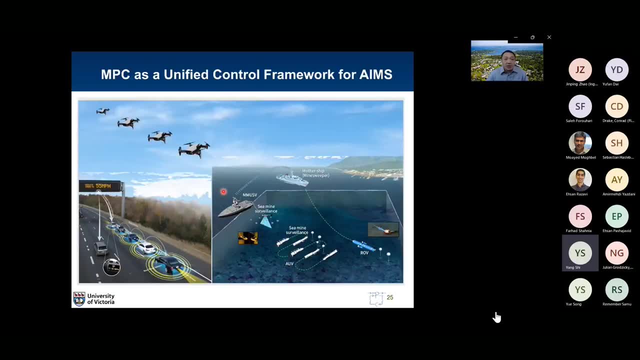 cooling, heating and power system. it's a it's application of advanced control and optimization to energy efficient systems. so overall our objective is to develop npc, that's, a unified control solution for advanced ai ms. so including the application of npc to drones or a group of drones as a team to autonomous vehicles. 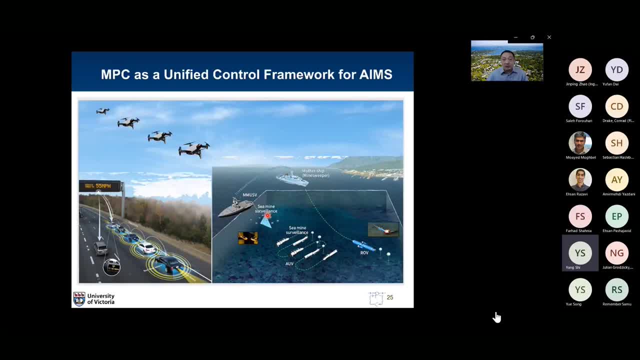 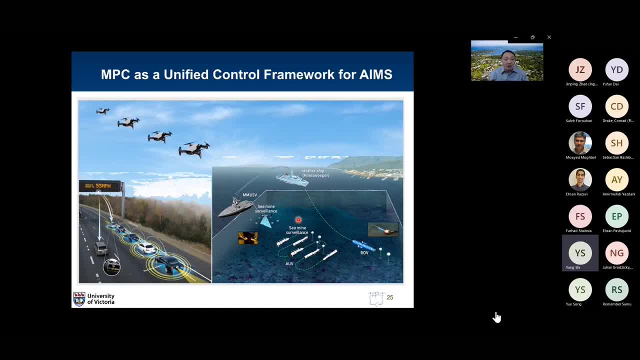 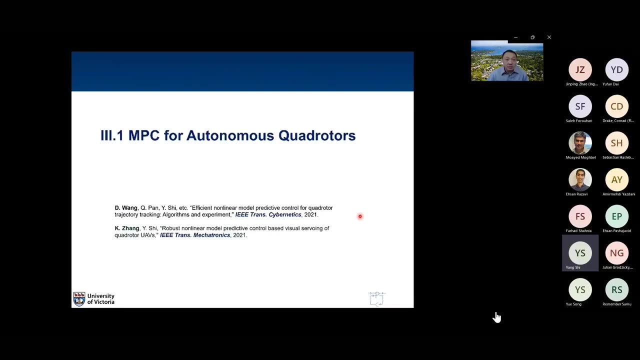 well. so mpc. due to its various flexible optimization structure and configuration, it can be potentially regarded as a unified framework to implement the representative dynamic systems. So the first work is on applying MPC to autonomous quadrotors. So we recently published two papers and several others. 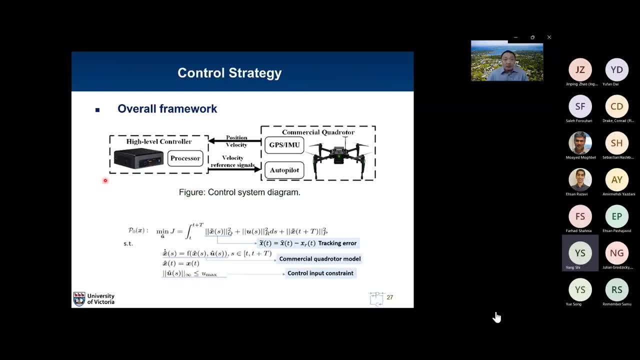 So in this work we need to implement the tracking control in the real system, real flight system, And then we have the high level controller to run the optimization based MPC. And then we have the sensors, GPS, IMU, equipped with the quadrotor to provide the feedback position. 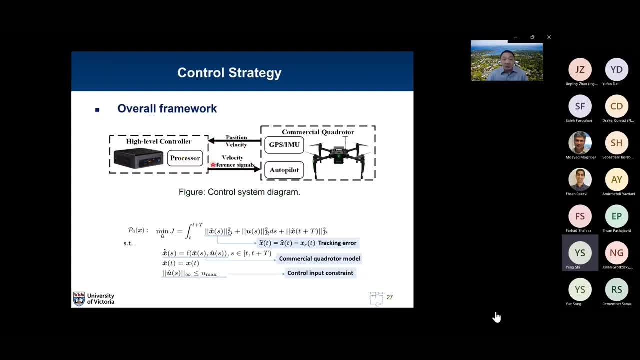 and the velocity information And then we send the velocity reference signal to the autopilot on the quadrotor, So formulating the problem as an MPC setup. So we see that the cost of function, So it will incorporate the tracking error into the cost of function, 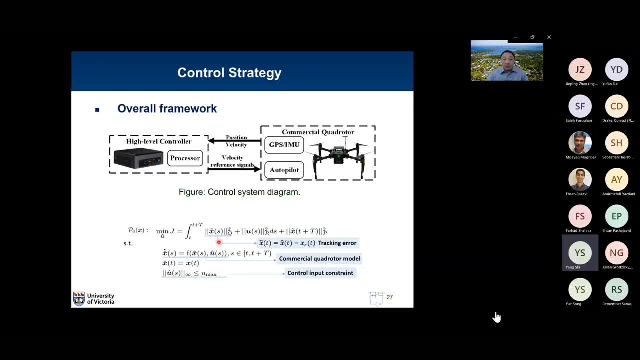 And then the first two terms are very similar to the traditional L4. QR control quadratic cost. And then the third term is added. here It's called the terminal cost to achieve the stabilization, to achieve the stability for the closed loop system. 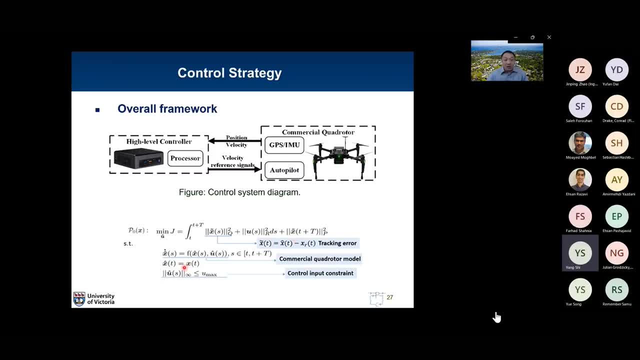 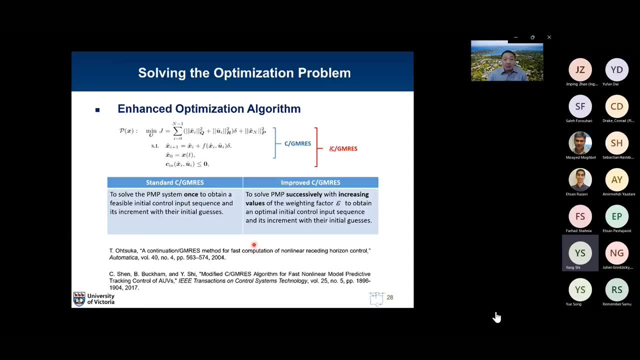 And then all the constraints can be added into the constant optimization problem. So we see that here the real challenge is to develop a fast optimization solver or algorithm to solve the constant optimization problem Within the very short period of time. So, based on the previous work on the CGMRES algorithm, 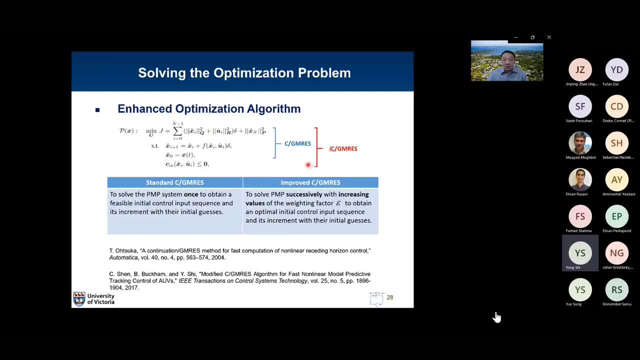 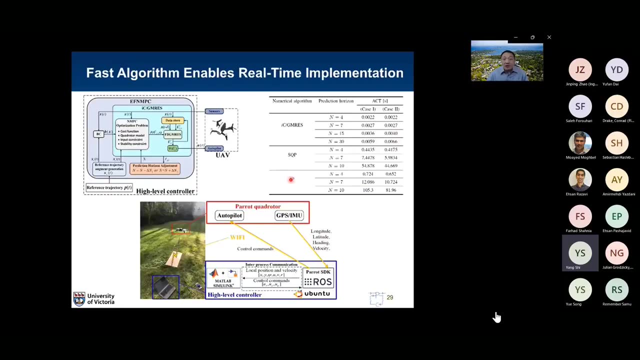 we further developed the enhanced algorithm to specifically deal with the inequality constraints, Because in our application inequality constraints are always encountered and need to be incorporated. So we can see how fast this new algorithm can achieve So, compared to the traditional classical solvers of SQP and IP. 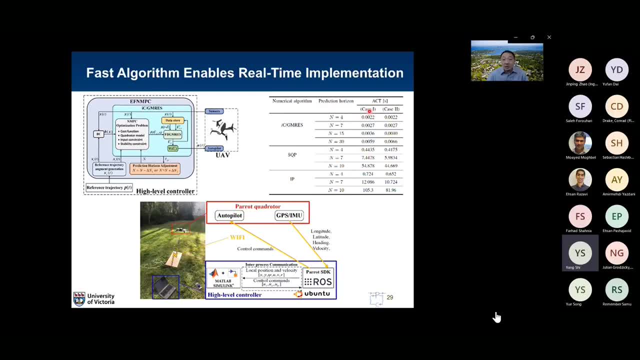 algorithms. you can see that in both of the cases. so our proposed algorithm can solve the problem within 0.0022 seconds, which is a significantly increased speed. So this capital N refers to prediction steps. So even by increasing the prediction horizon to be 30,. 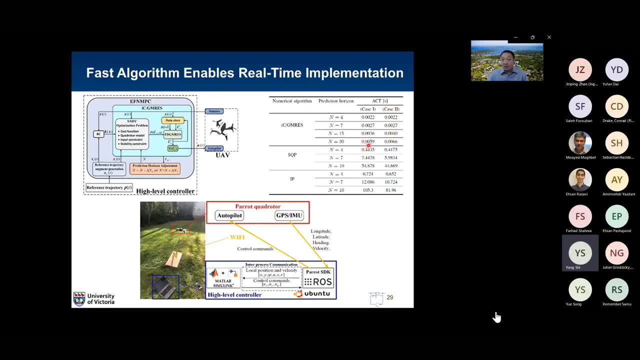 so we can still solve the problem within 0.006 seconds. So this can very well successfully enable us to implement the algorithm in the real time flight. So the flight path showed us that the tracking performance can be satisfied very well. So, as I mentioned earlier, fast implementation. 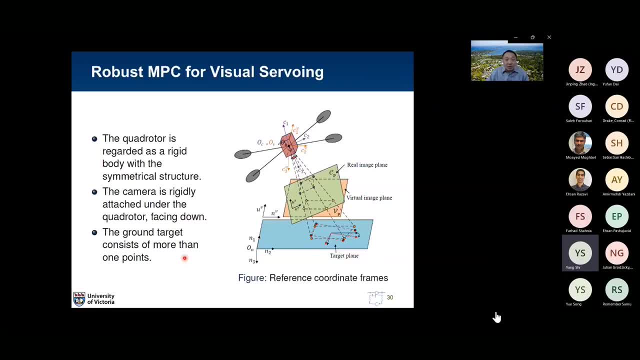 will be playing an instrumental role in applying MPC algorithms to any type of electronics applications. So this is a second example. We propose to integrate the visual serving with robust MPC. So if we have a drone equipped with a camera, so under the environment, without having the GPS signal, 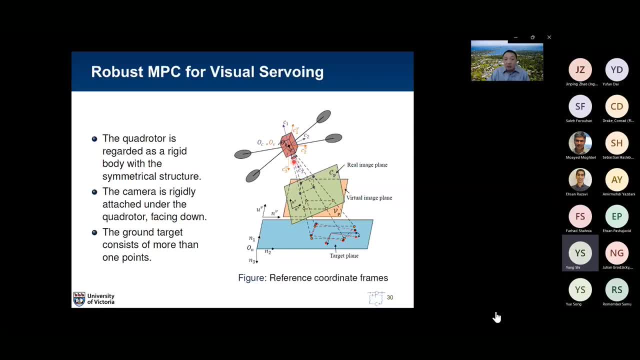 we need to make use of the visual serving images, information as a feedback. So in this case, our contribution lies in that we propose to include the visibility constant into the MPC. So, again, this is due to the flexible optimization structure, configuration of MPC. 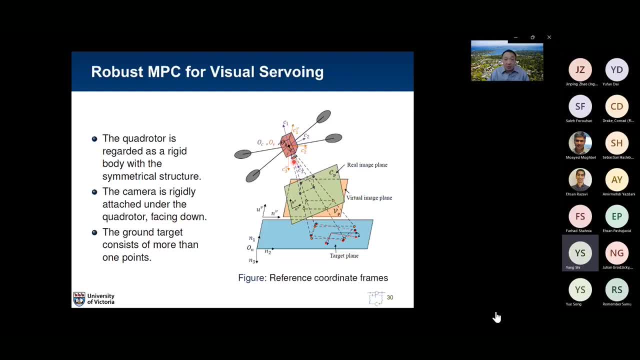 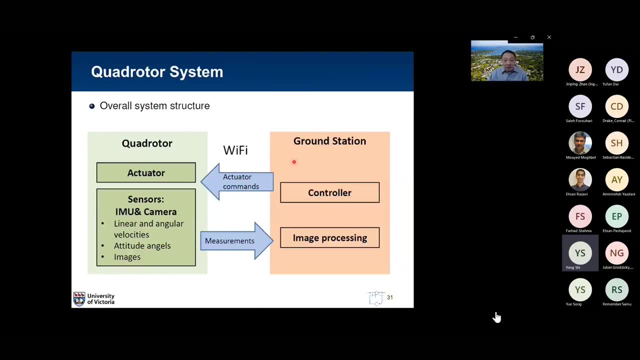 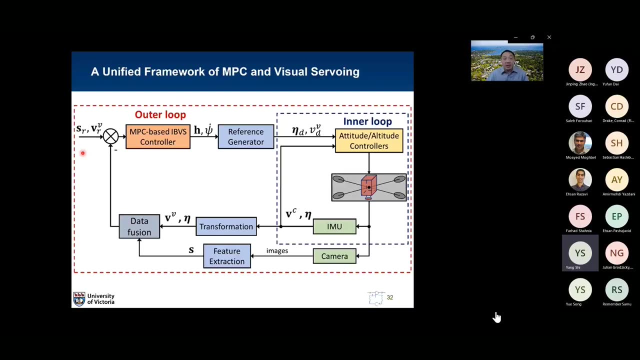 We can incorporate many practical constants into this framework, So by incorporating the image as a feedback, and then we can implement the flight control for the quadrotor. So this has been designed in terms of two loops, as many others quadrotors are implementing. 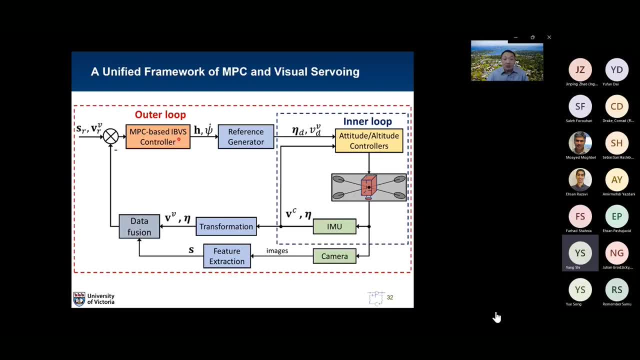 The outer loop we are using the MPC-based image-based visual serving controller And the inner loop it's implementing the local PID-based attitude and altitude controller. So the connected visual information will be sent back over internet to the controller. So the controller will be operating and solving. 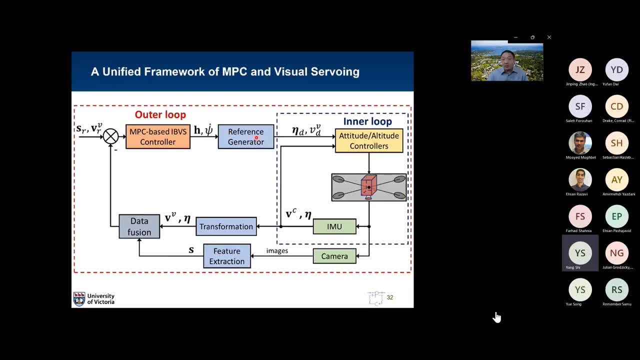 the opposition problem and sending the commands to the quadrotor to implement the tracking objective. So under this unified framework we can see that not only solving some traditional problems, control problems, if we have a new requirement like including the visual serving into the system. 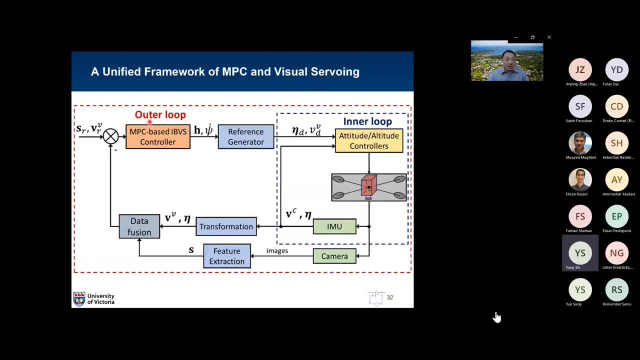 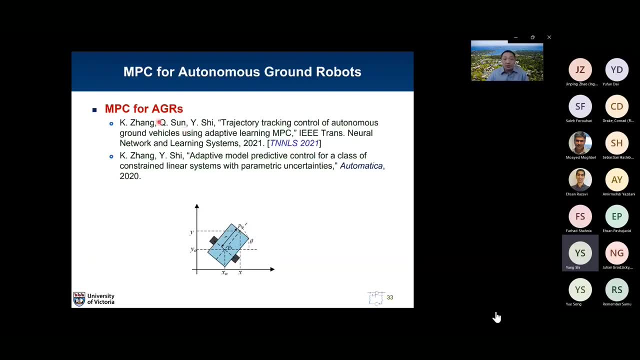 so MPC as a unified framework can very conveniently and systematically provide a solution. We also apply the multiple PID control to a type of autonomous ground robotics, the two-wheeled ground robotics. So in this case we specifically focus on solve the problem on. the mathematical model may not be always accurate. 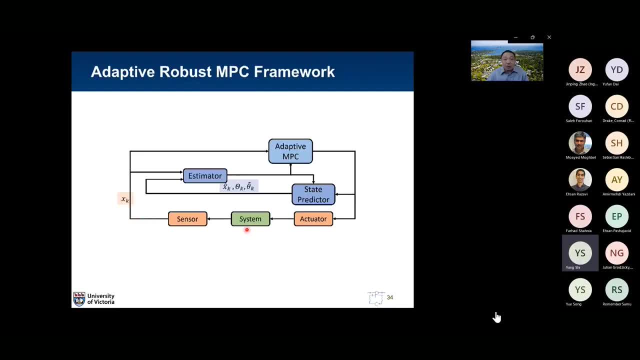 and precise enough. So in this case we need to propose the so-called adaptive and learning robust MPC framework to tackle the problem, Because in many applications the mathematical model is a way or has discrepancy compared to the actual physical system. So in this case, the adaptive MPC is 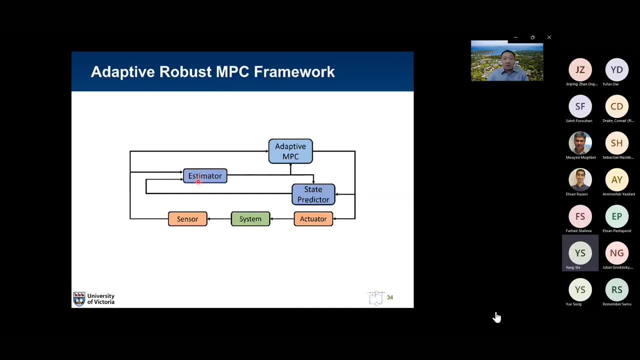 a more robust MPC. So the MPC strategy will incorporate an estimator to online identify the model parameters And then the update in the model will be used to solve the opposition problem, leading to the adaptive MPC framework. So here, in order to further enhance the performance, 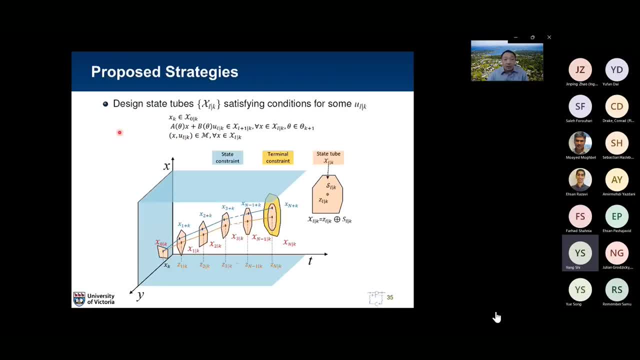 of the learning or adaptive-based MPC, we need to incorporate the robust strategy like the two-based MPC. So from this figure, so sorry we don't have enough time to introduce in more details, but in general the idea is even there. 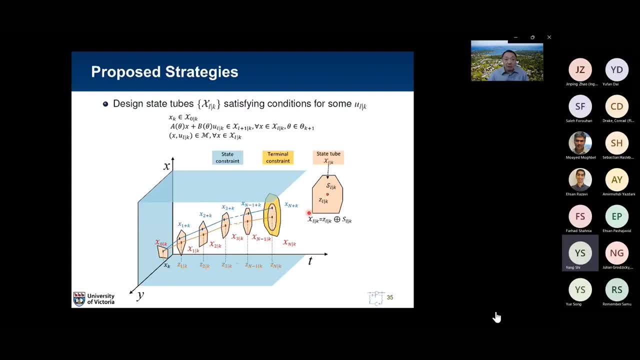 will be some uncertainties exist and disturbances introduced to the system, And also, even though there will be some estimation error or identification error on the parameter, say that to be estimated. so considering this estimation error as a certain type of disturbance to the system. so 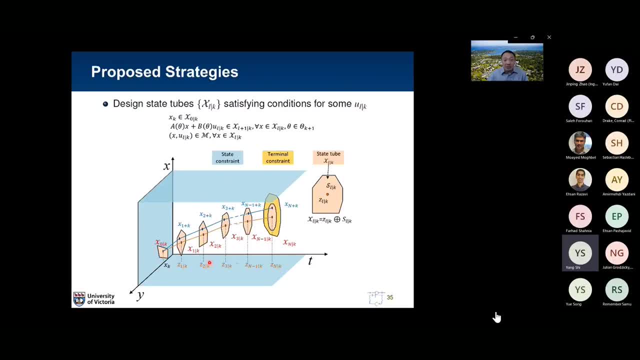 we are going to design the adaptive and the robust MPC to be still able to tolerate towards against this estimation error. So the way to tackle this is to design some tubes as shown by these figures and then, as long as the disturbance will be within certain level, not exceeding the worst case upper 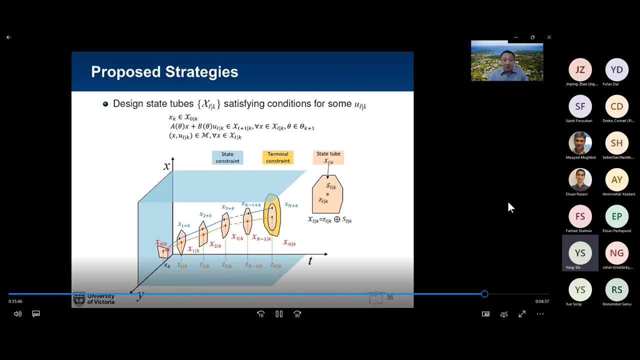 bound. we can always guarantee the generated stage trajectory to always remain within this tube as described. So this needs to further adaptive learning based on robust MPC strategy, which suits very well for the needs of the mechatronics applications. So this is a resorting constant. 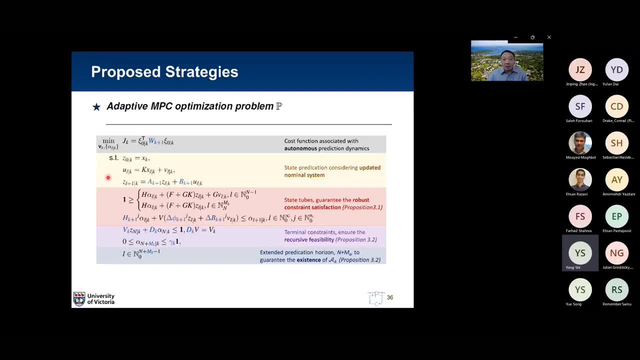 optimization problem. and then you see that not only we incorporate the current estimation into the scheme, but also we introduce some state tubes, new tube methods, to enhance the robustness of the proposed scheme. It can be generalized to be applied to many types of mechatronics, dynamic systems. So this is a 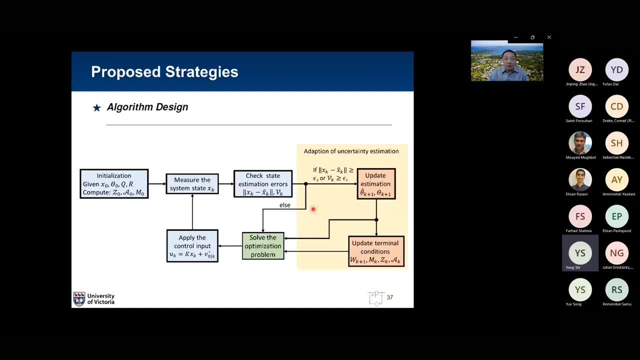 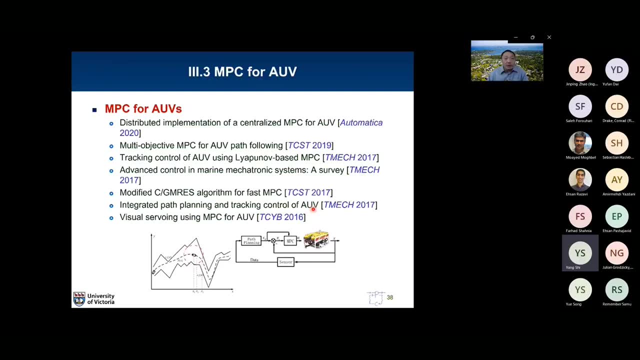 algorithm description for the experiments and experimental and simulation results showed the effectiveness of this type of method. So, finally, I'd like to very briefly introduce our some applications of model predictive control for autonomous underwater vehicles and autonomous surface vehicles- marine applications. So in this case, not only we are going to solve the tracking control. 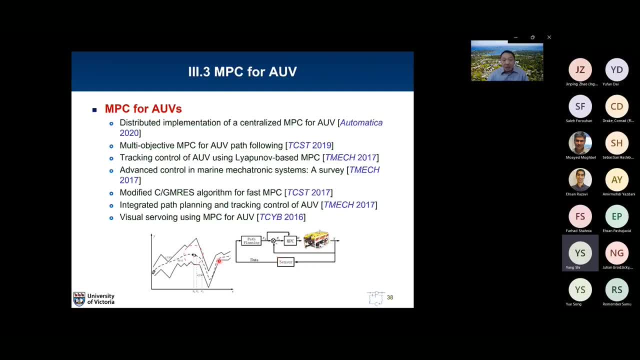 for the vehicle itself, but also we can incorporate the path planning into the optimization framework. So just to recall that MPC is an optimization based strategy and path planning is also an optimization based procedure and we propose to have to design an integrated optimization framework for dealing with the path planning and further the tracking or path following. 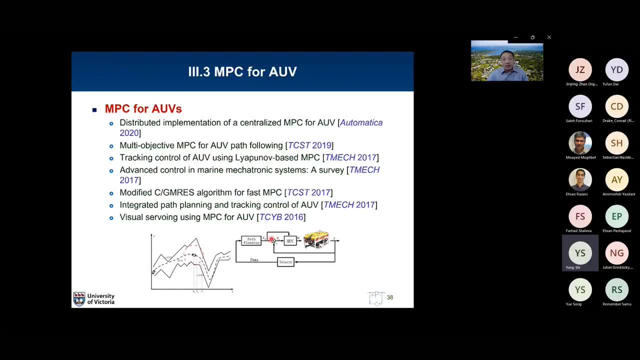 or dynamic positioning and so on. So this way we can- we can regard multiple control as a unified framework to deal with the related engineering optimization problems. And in addition to this, we have developed some other type of MPC strategies specifically for the underwater vehicle applications, like the path planning or how to improve the implementation efficiency. 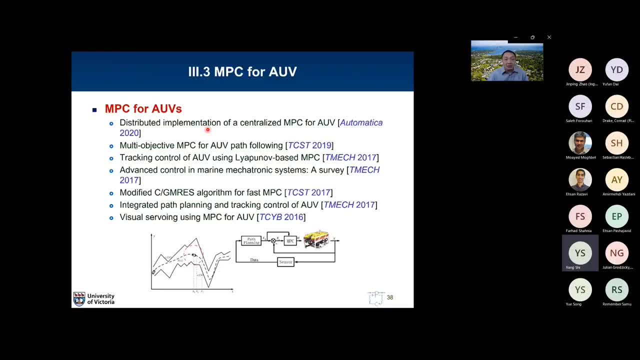 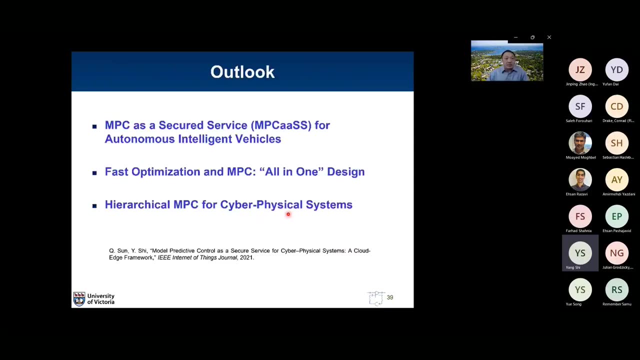 increasing the solving, the optimization problem, speed and also to provide the visual serving into MPC for underwater vehicle applications. So this gives us the brief summary of today's talk and in the future we believe that MPC should be developed towards a secure service for autonomous intelligent vehicles, So secure. 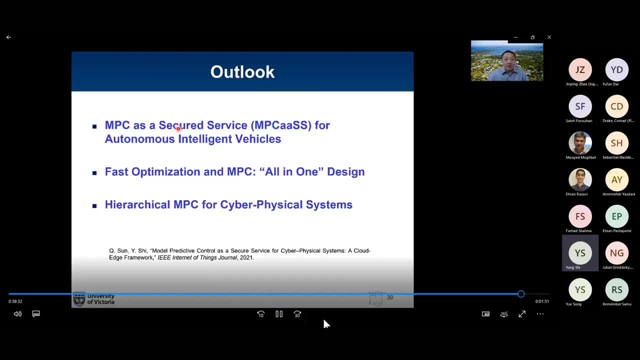 requirement comes from the cyber physical system setup in any of the application scenario of future electronic system into the cyber and physical domain interaction. So security will be an important issue we need to offer And further controller design may not be, you know, always following the traditional engineering philosophy. In the future controller design will be a type of 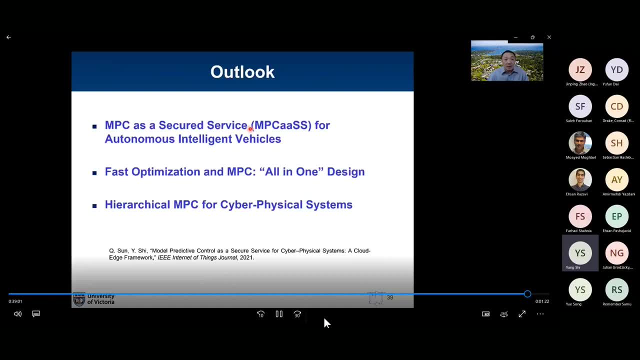 a service provided to our industrial customers. In terms of the tactical development, we aim to integrate and combine the fast opposition algorithms together with a dynamic controller system design analysis, so that's a so-called or in one design. so currently, you know, researchers are studying. 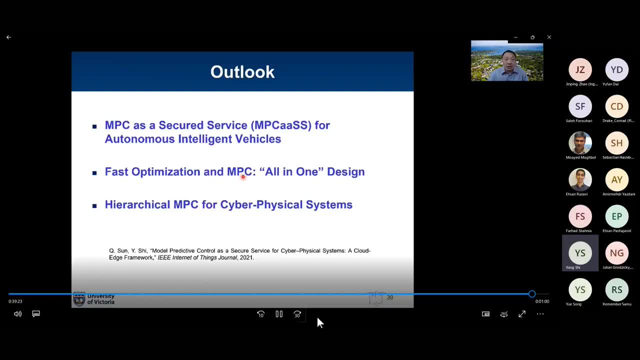 optimization and some others are focusing on controller design. however, they are actually just uh in one umbrella and hierarchical npc for cyber physical systems. that's my uh, that's our ongoing research direction for dealing with a large scale cyber physical system. we have to propose a hierarchical structure for modeling the large scale system and then accordingly provide a 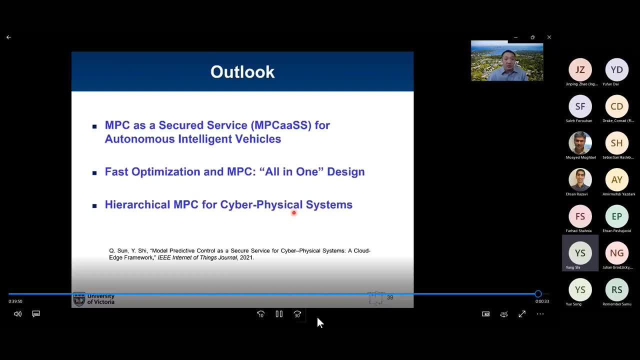 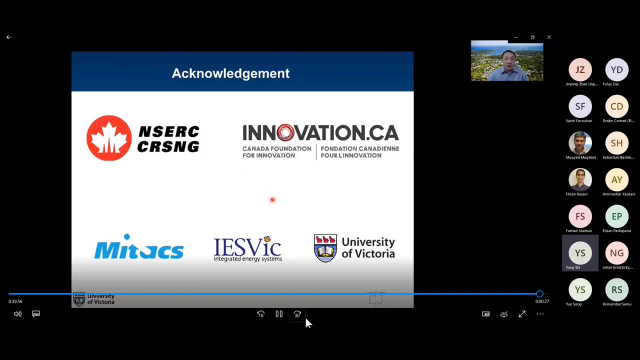 solution to design npc for such a hierarchical, large-scale cps system. so this is the end for today's talk. i'd like to quickly acknowledge uh funding agencies supporting our research, including insert canada foundation for innovation and metax, and university of victoria ice fake institute of the 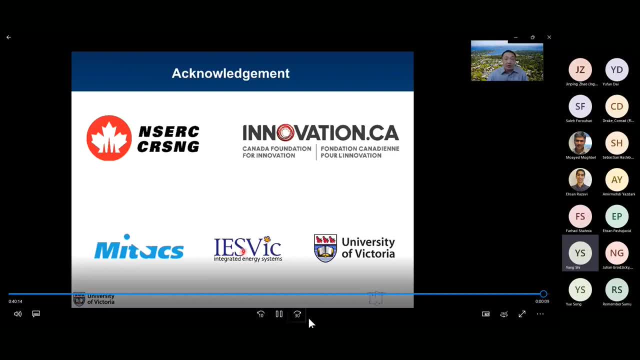 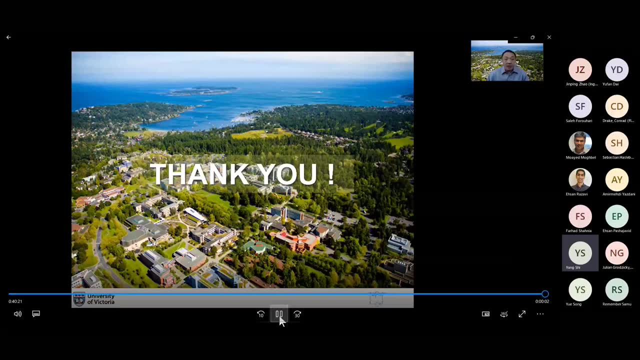 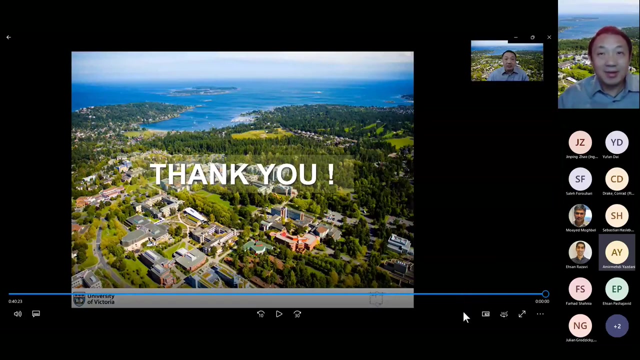 energy, integrated energy system and many other collaborating companies and industrial partners. thank you so much for your patience. i would be very happy to answer any questions. thank you very much, professor xi, for your very interesting, insightful presentation. i enjoyed a lot. so it's time for our audiences to ask their question. please feel free to ask your question. 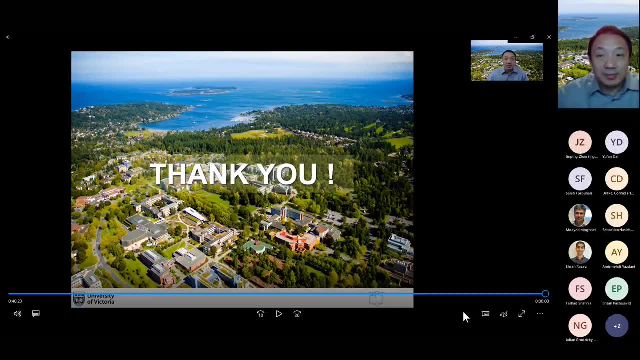 thank you. i've got two questions. if yes, please. so yeah, essence here from ema. so thanks for for the presentation, very interesting topic. um, i've got two questions, uh, the first one is: what's the normal time interval for each step of npc in robotics applications? 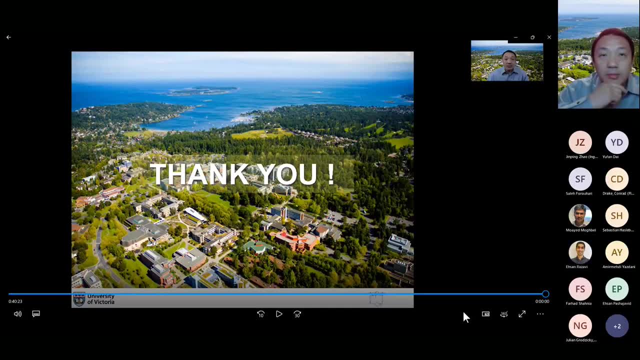 i'm just curious to know, uh yeah, so, uh normally, if you are uh talking about the flight control of quadrotor, so normally we operate this something period at uh like 0.01 second, i believe. for robotics application it's a, it's almost at the same level, or sometimes 0.001 second for faster dynamics of. 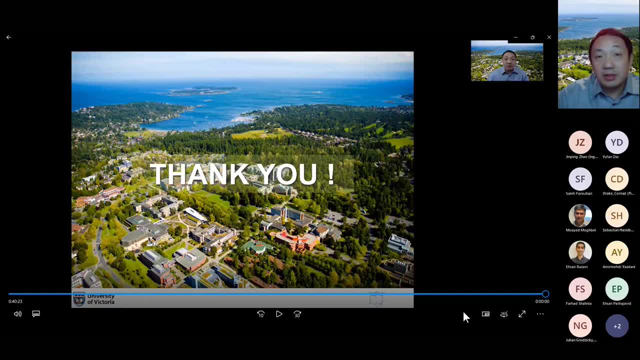 motion control systems. so therefore, uh, even though npc model predict control has found- you know very uh you know- successful applications in process control system, like uh oil industry, uh process control, because those systems are of a rather longer sampling period. so solving the optimization problem uh would not be a concern but for robotics application in order to implement mpc. 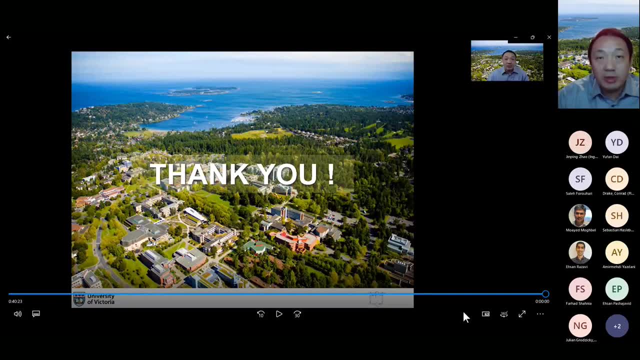 uh, you know, the first uh bottleneck problem is uh to find out a very efficient solver for the formulated optimization problem. but in the past five to ten years, robotics areas, motion control systems, are applying npc, you know, according to the report from some robotics companies, and also autonomous driving applications. 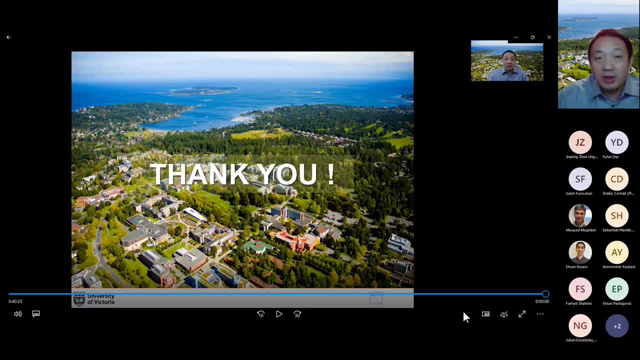 see uh many reported results on on the successful application of a model predict control. yeah, thanks uh, i think that's a very short period of time in terms of the interval. so, yeah, the fast npc would help and i guess the linear uh optimization would help a lot. and 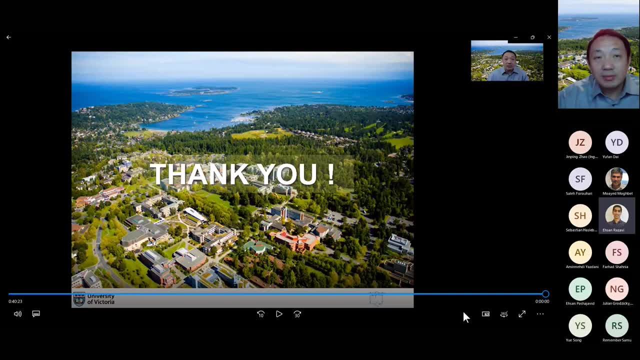 here. my second question is depending on on the time interval of the case. so we could have some observation to shrink the horizon to to fit in the npc model for the, for the next time, for the next interval. so definitely, as you said, there could be some delays or even the cyber attacks. 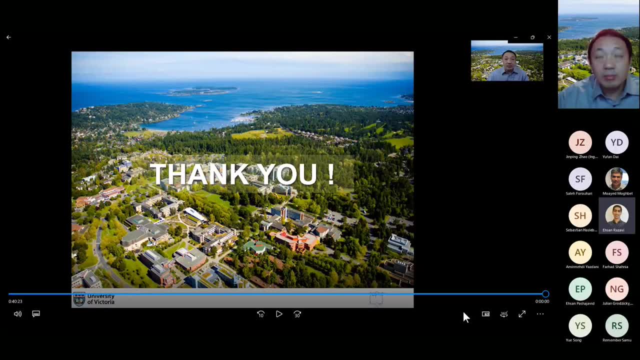 to alter the inputs or even the loss of comms. so how do you think the estimate, the auto estimate, potentially coming from out of the in npc model, could be integrated in such applications to improve the the performance of the control model? i'm i'm actually talking about another layer of estimator. 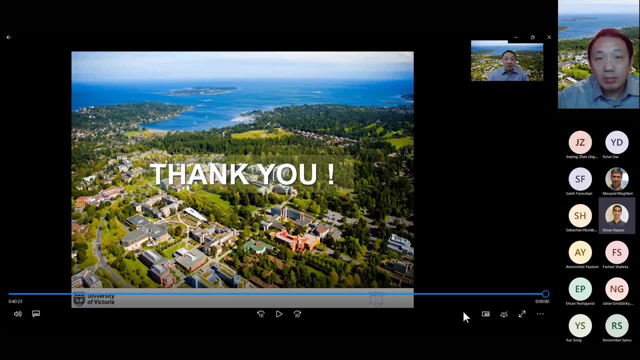 if, if you just go back to your slide 34, probably so- there's a estimator over there and in such applications if there's the delays significant or the loss of comms. so do you think another layer of estimator or predictor can help or is there any work has done? 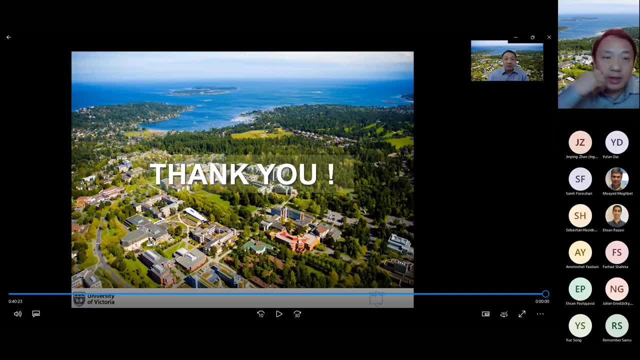 in this space, uh, yes. so, uh, when we're talking about the uh model accuracy, i think it plays an instrumental role in determining the actual performance of uh application of npc. uh, normally, uh multiple control assume that the model is uh perfectly known. uh, and the model is perfectly known. 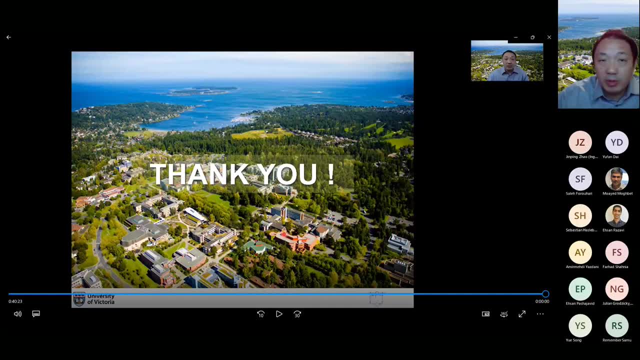 and then in the next uh step we apply the robust npc. considering some uncertainties and further in our work, we have been working on developing the robust and adaptive npc by integrating the estimator, as you just mentioned. so if we incorporate the online system identifier or estimator to try to update the model parameters in real time, so this can uh you know further in. 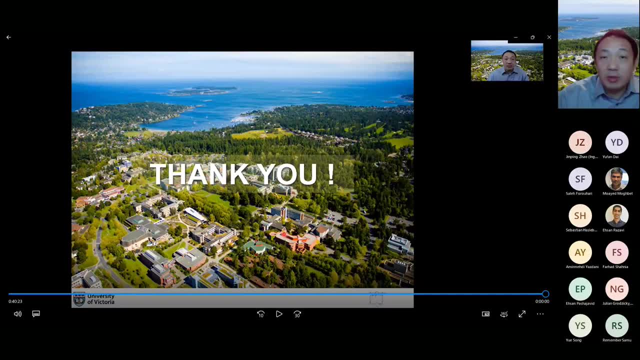 house the adaptivity of the scheme towards the parameter uncertainties and also further if we have, uh, even unknown non-linear functions, that's involved in the model dynamics. so we can introduce a learning based approaches like reinforcement learning or some other type of approximation using neural networks to enhance the online estimation approximation of the adaptive. 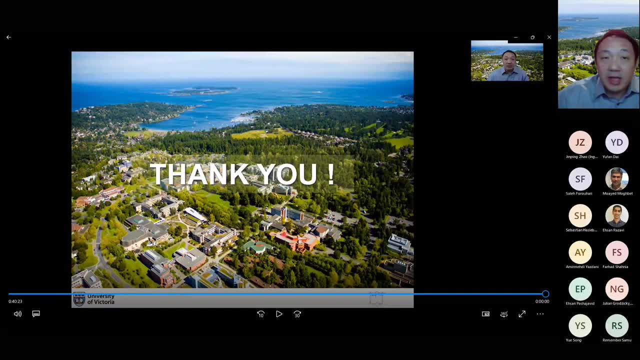 control. so i believe, uh, you know, adaptive and then learning, a multiple control will be very important uh in dealing with the inaccurate mathematical model. thanks, yeah, sure, and i think i think, in terms of the real-time uh applications for, for the adaptive control, if, yeah, i understand, so we get, we look at the real-time data. so if we lose some of the 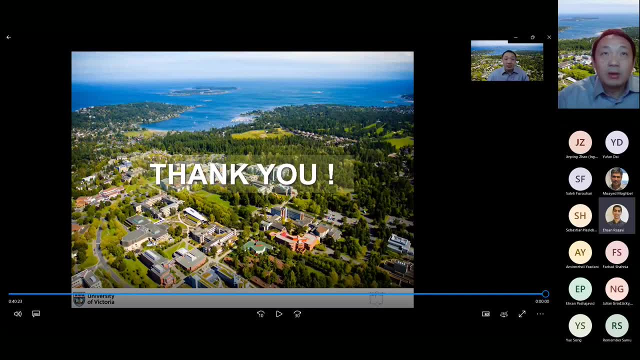 data. so what are the backup plan for that? i mean, if we've got any estimators other than, you know, the basic one in the npc model, do we- um, you know, does he have any any other model to to estimate it? or it's the same model, but we're trying to for those periods of time, we're trying to return the 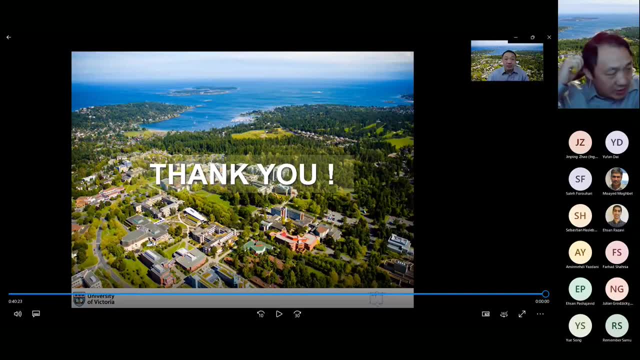 same model? uh, that's a very interesting question and very insightful question, uh, thanks, uh, i think, in reality, definitely, as shown in the one of the previous slides. so when we're connecting the data from the wireless communication channel, or even from local connection, or measurements of the of 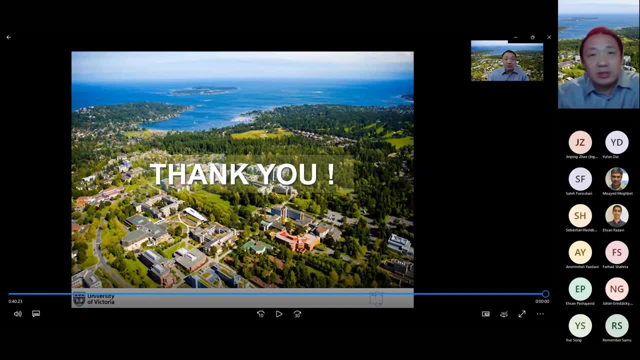 the data. so we may uh subject to some data packet dropouts, right, so this needs to sometimes a random packet dropouts. so in this case, we need to provide a online estimator dealing with this uh intermittent, uh information loss. so so, in this case, uh, thanks to the npc's feature, because npc 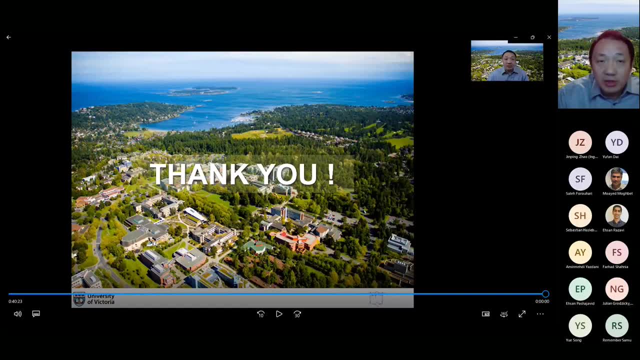 can do some prediction of the state information. so if, during the measurement of the state information using some sensors, the data will be lost and then we can make use of some- uh, the predicted state from the mathematical model of npc to to provide a compensation to some extent, so we ever studied this type of methodology or approaches. 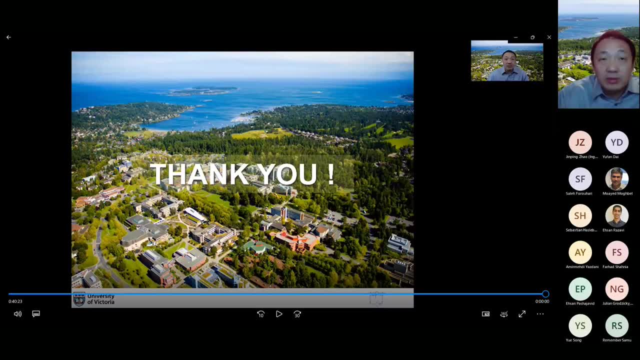 and then incorporate this idea with the adaptive control to try to enhance the estimation identification of the model and, on the other hand, so another research idea or frontier is to incorporate the model predicted control with the digital twin, a magneton when running the model predicted control in real time, we can also operate the digital twin model. 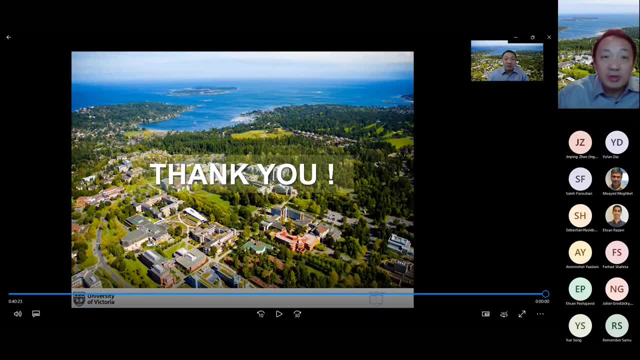 hopefully the model can simulate the true system as close as possible. in this case, if there would be any uh information loss or due to some deal as a pack, so this digital twin model can provide some compensation. so in this case definitely this compensated the signal for the missed data. 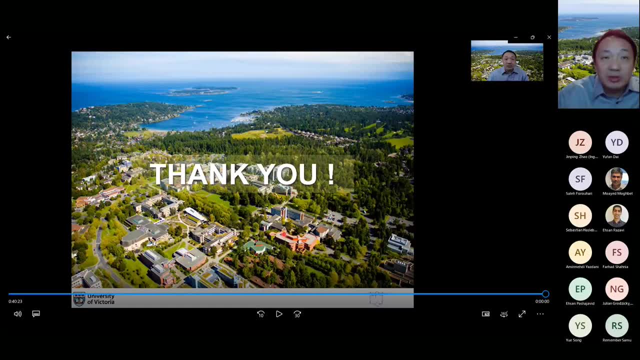 is has a discrepancy compared to the true data, but we can use some robust control tactic to try to suppress the negative effect due to the mismatch between the compensated data information versus the true data and information. so therefore, adaptive and robust mechanisms are closely collaborating together, providing uh the satisfactory performance. 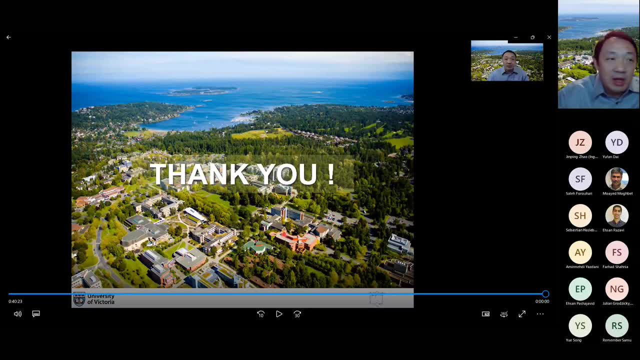 so, in summary, if there would be some information, uh, intermittent, uh, uh miss or or loss, so theoretically we still can find and develop some algorithm to make the compensation. yeah, thank you so much. thanks so much, professor yep, that's me. thank you, professor shi, for your answers. is there any other question? 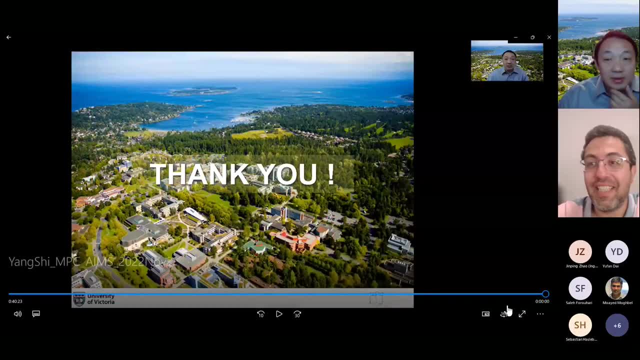 uh, yes, may i have one question? so first of all, thank you, uh, thank you very much, professor shi, for the excellent talk and very good to see you again after such a long time. uh, thanks, it was a very excellent talk. my question is mainly about the topic of distributed npc, which you gave some 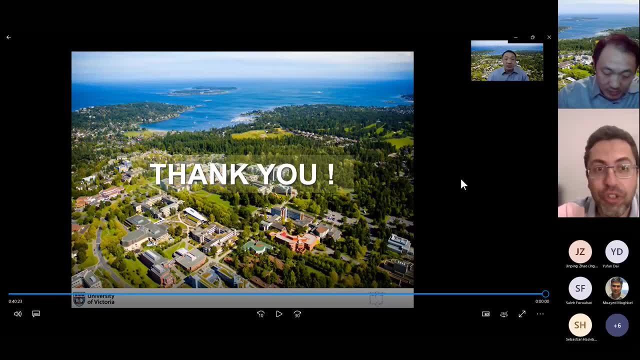 examples, for example with the uh cars. do you think how much we are far away from having really cars driving autonomously using this distributed npc control technique, or do you have any knowledge about the industries that are testing or implementing these things? uh, so, thank you. thank you for the very nice question. uh, yeah, same here. uh, very exciting to. 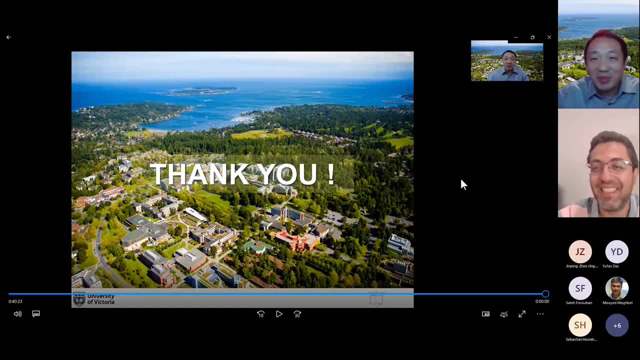 to see you again online. hopefully we can meet with each other in person in the very near future. regarding regarding the distributed implementation uh, from the theoretical side we have a developer from uh distributed the robust npc uh methods for controlling a multiple agent system including the vehicle plateau or asv autonomous surface of vehicle plateau. uh setup uh and in experiments. 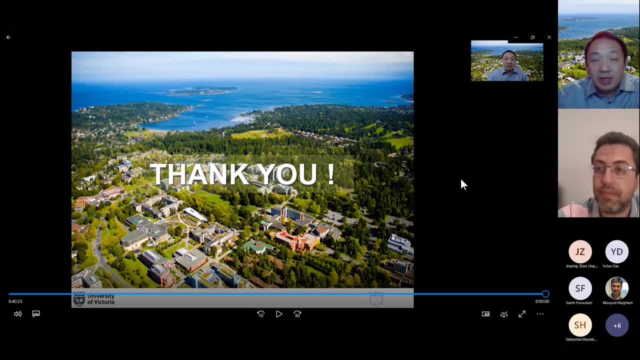 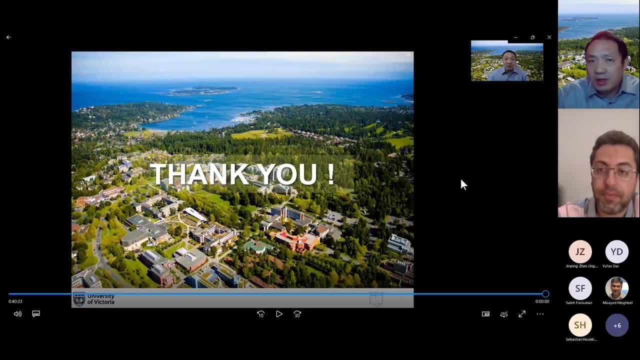 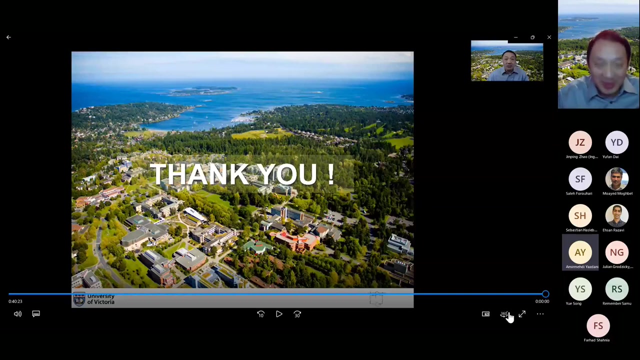 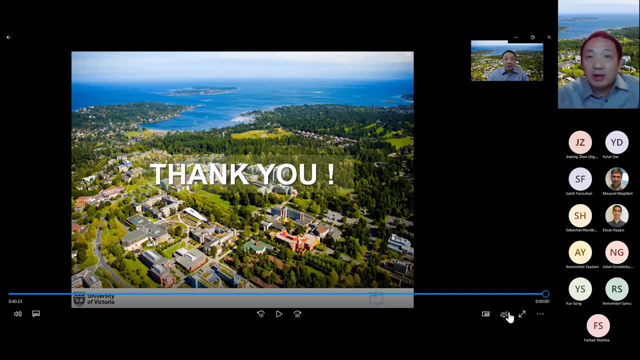 an insightful investigation of a theoretical study on model predictor control. So, because a model predictor control is an optimization-based method and it's performing the solving the optimization problem every periodical time, So it's a receding horizon magneton, So every fixed period of time we need to solve the optimization problem, generating 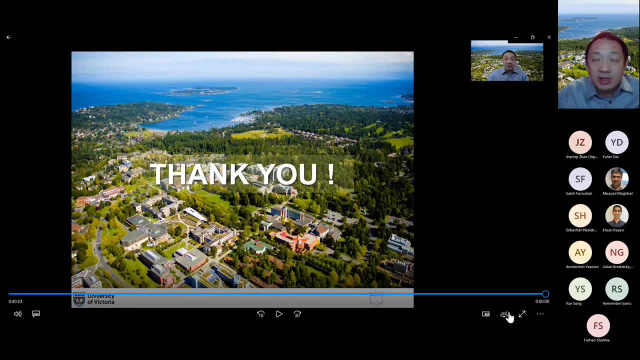 the control sequence. So therefore generally the generated control input signal is kind of a numerical solution. So therefore this poses some challenges and difficulties in analyzing the closed-loop stability by picking up the first element of the generated control sequence or profile for implementation. 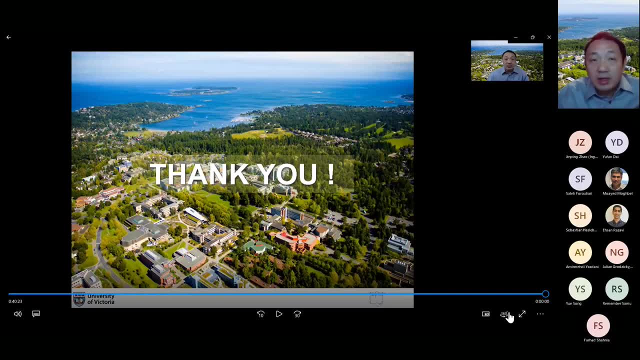 So therefore, I think so far in our theoretical study, we always try to provide some necessary conditions. Under these conditions, we can guarantee the stability of the closed-loop system. So, generally, normally, in order to achieve this, we need to do something on formulating. 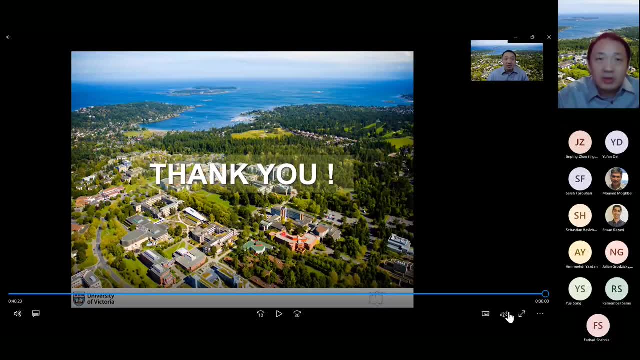 the optimization problem, For example number one, we need to add an additional cost, called the terminal cost, into the objective function. So this terminal cost will perform, will serve the need of the object And this terminal cost will serve the need of the object. 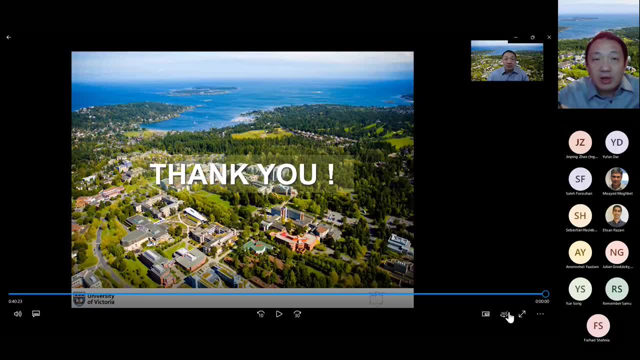 And if we do that then we can get the value of the proof for feasibility and stability. And also we need to add a constant. This constant is on constraining, that's a terminal state, So in general we can have the state constant. 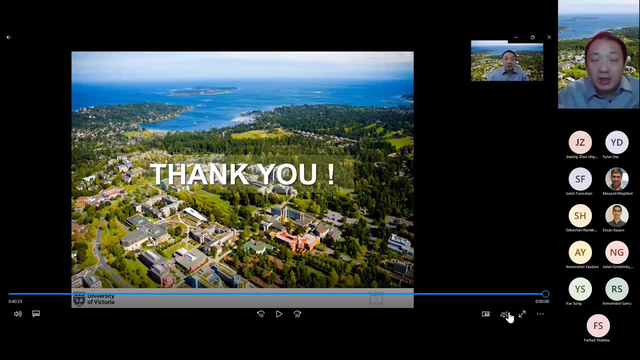 We can have the control input signal saturation constant, but in addition we need to normally add a constant on the terminal state. Terminal state refers to the last time instant of at the end of the prediction horizon. that end we need to put a constant set on this state specifically. so by having both of this, 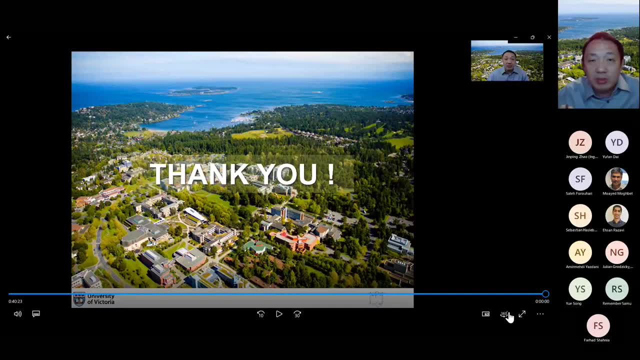 added additional requirements to the formulated opposition problem, we can successfully prove the feasibility and also the stability of the system and, interestingly, when ensuring both of these important properties, we end up with establishing a set of conditions. so these conditions in the paper may look very complicated. however, they are closely related to some physical 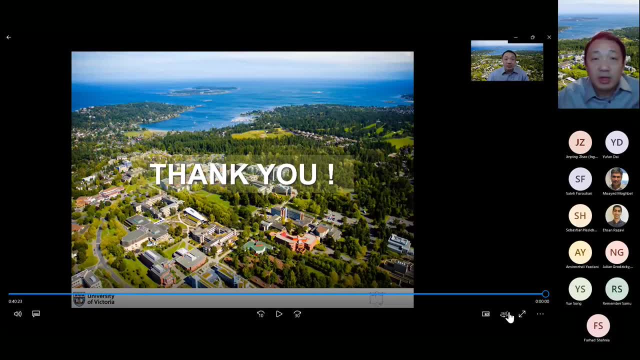 parameters in action for implementing the controller, for example, feasibility, meaning that the opposition problem must provide a feasible solution. so it depends on the choice and design of the prediction horizon. so what's a length of the window for prediction? in theory, ideally it's a longer. the longer the better. but in practice it may not be the case, because the practical 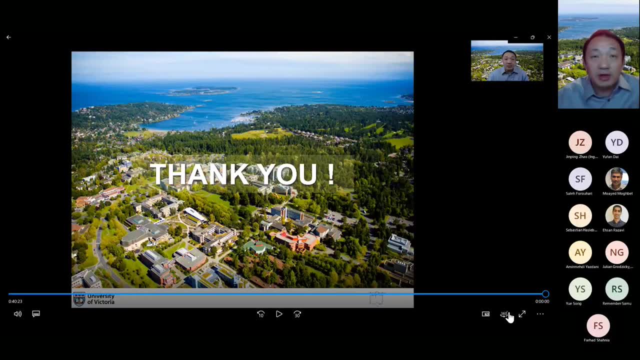 application will be subject to some uncertainties. if you make a very long prediction, considering the uncertainties, this prediction may not be accurate because it's disturbed by uncertainties. so therefore the condition will be reflecting the dependent relation on the prediction horizon choice and also the sampling period- how long time we are going to. 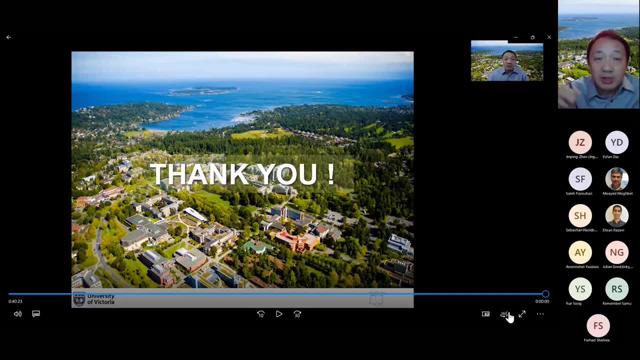 do the optimization. so this is called sampling period. so this parameter is also determining the feasibility and the stability of the closed loop system, and also we have some other parameters to be designed. so all of this will be reflected from the established conditions for ensuring the theoretical properties. so i think, regarding the theoretical analysis, we can find the ways to 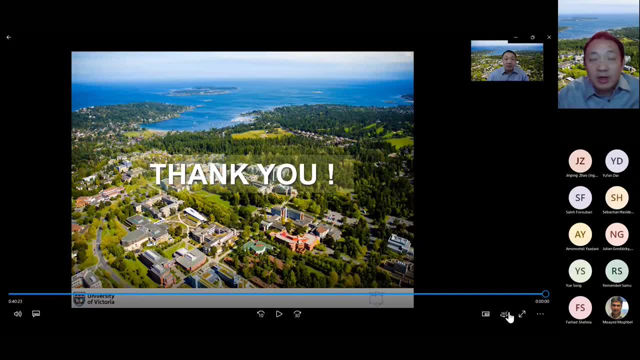 to always theoretically ensuring and proving these two properties, and theoretical study can provide guidelines for doing the test for realizing this algorithm in real systems, because they provide a range for choosing their parameters. so that's my brief answer regarding the theoretical study on MPC problem. thank you very much. it was really comprehensive and detailed answers, you know. 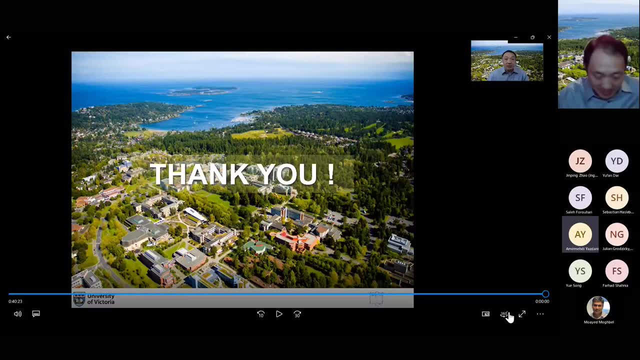 considering all aspects. so my second question is: uh, just to know your- uh, you know- recommendation for the off-the-shelf software you know, uh, that's uh include the- you know- MPC technology. there are many, you know, like Akadu toolkits or Kassadi and so on and so forth. i'd like to know with which. 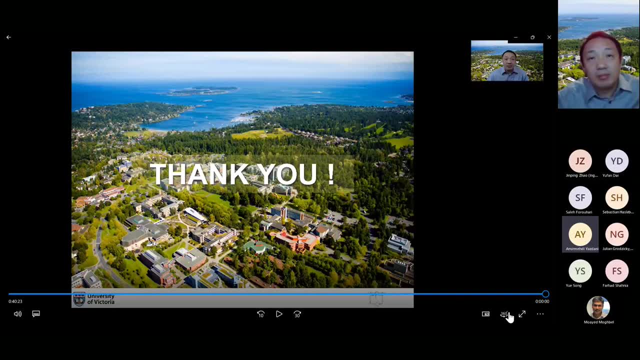 one is more convenient for the user and facilitate the ease of implementation. uh, i think, uh, for a theoretical study first step, we need to do some simulation study to verify the algorithm. so sometimes we use a MATLAB fmincon function to solve some optimization problem, and Kassadi can also be used and yallet can be used. there are some open source solvers. 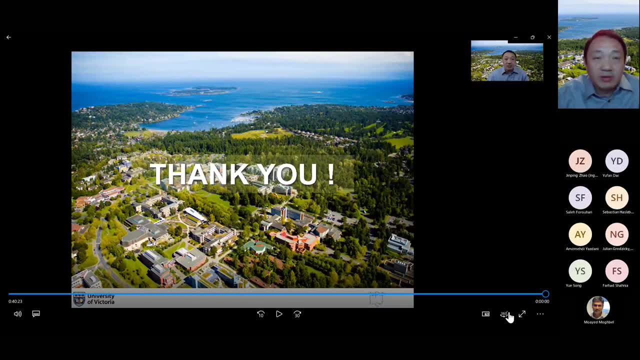 and also we ourselves, uh also you know, develop some optimization algorithm, it in the paper, and we also make it uh open source, uh, so, uh, it's a, it's open source on github, uh, i think, for real-time implementation in. in that case, i think we need to be very careful to choose. 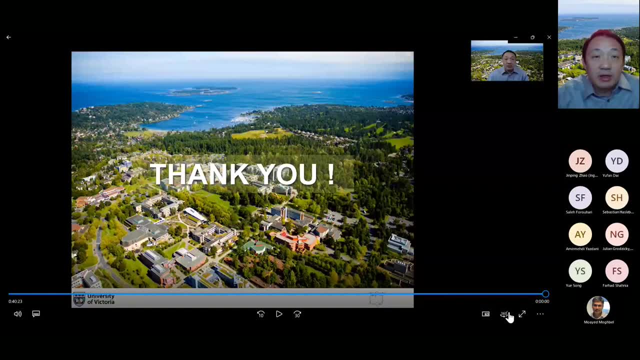 the very suitable solver that can provide the capability of the solving the formulated optimization problem within the short period of time for motion control system. but because most of our works are in the lab-based experiments, so the mentioned solvers can can serve, uh very well. thank you very much for your answer. is there any question? 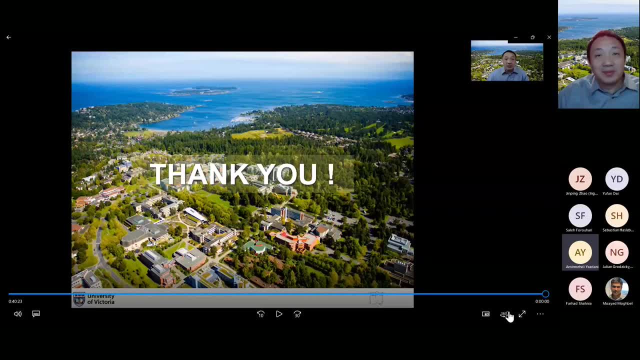 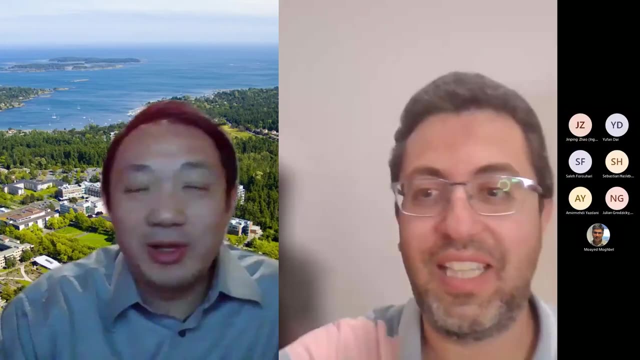 okay, it seems that there is no more question. thanks a lot for accepting our invitation and for your fantastic talk. we hope to see you in our next uh, you know, or next year webinars as well. sure, sure, thank you so much uh for everyone. uh attending this uh event- fabulous, and thank you very much for your for. 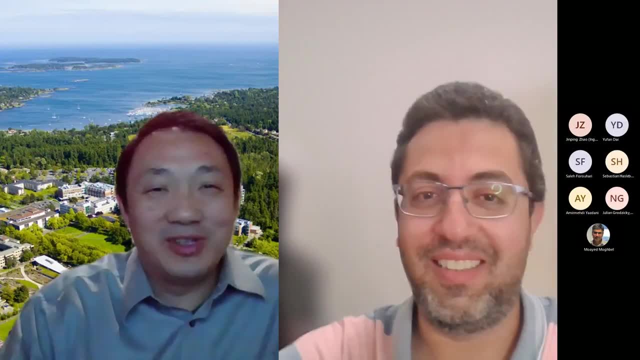 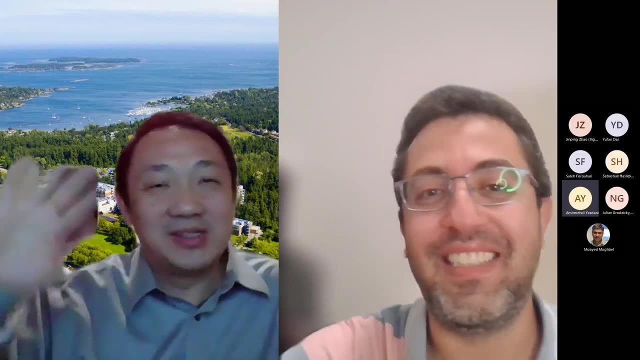 your invitation and yeah, we keep in touch and hopefully see you soon in person. thank you very much, thanks. thanks everybody for attending this webinar. see you later and have a good time. see you later, bye.